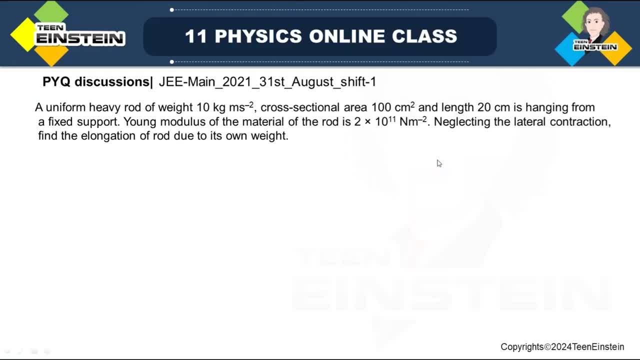 This conference will now be recorded. Very good morning students. We have been discussing PYQs from JE Men's papers, So today we'll be discussing PYQs from JE Men's papers. So today we'll be discussing- Excuse me, So yeah, suddenly I got a call Anyway, so let us continue. 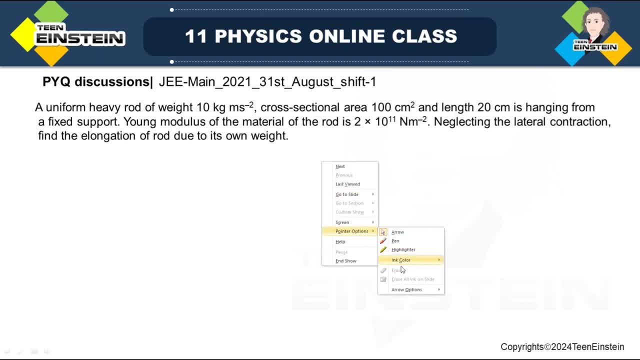 Let me change the ink over here. Okay, So today we'll be discussing questions from the 11th part, So from this particular question paper, 2021, 31st August, 6th to 1.. All right, So let us start our. 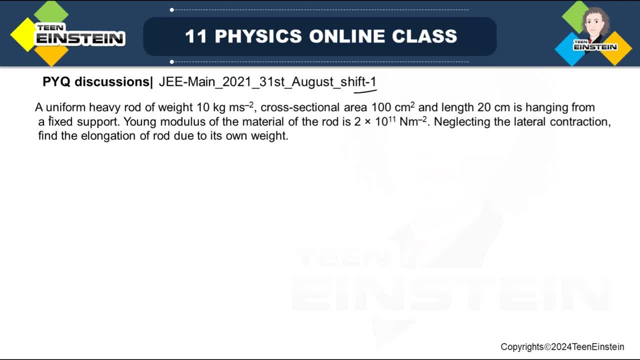 discussions. The question says a uniform heavy rod, Uniform heavy rod of weight, 10 kg Weight, 10 kg meter into meters and sorry, kg meter, second square. Okay, I hope you have understood this Kg meter. So actually the Newton is actually m into g in this case. 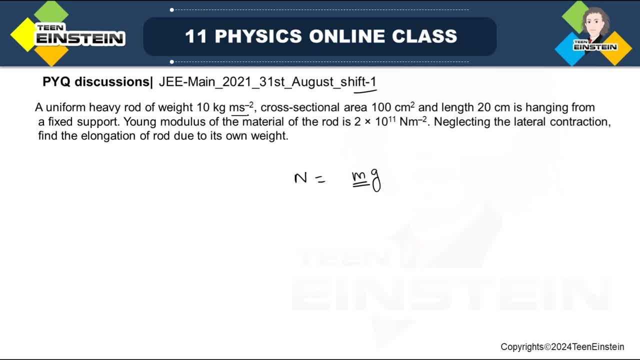 So it means m into g, So kg meter per second square. So in that way the unit is given anyway. So and the cross-sectional area has been given 100 centimeter square. The length is 20 centimeter is hanging from the fixed support. 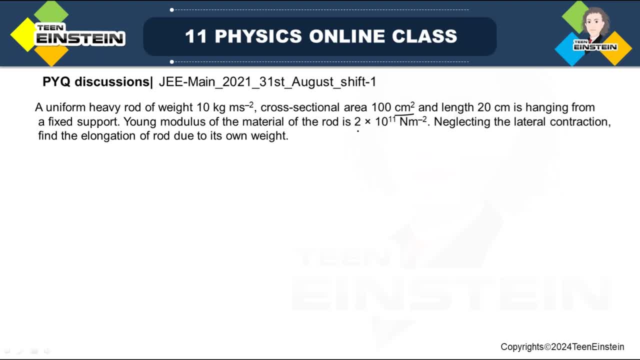 Okay, young modulus of the material of the rod is given as Two interchangeable 11 Newton per meter square, neglecting the lateral contracts, and find the elongation of the rod due to its own weight. Okay, So let me give you the options over here. 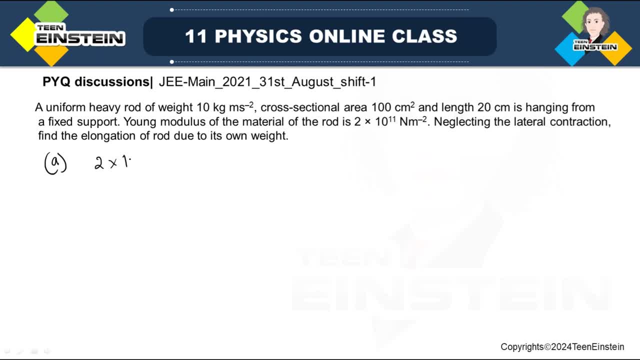 So option a is saying two into 10 to the power minus nine meter Kg meter per second square. Two into 10 to the power minus nine meter. option b is 5 into 10 to the power minus 8 meter and option c is 4 into 10 to the power. 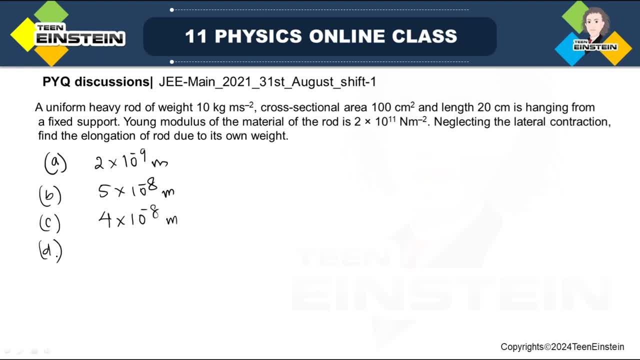 minus 8 meter and option d is 5 into 10 to the power minus 10 meter. okay, so the question is heavy rod. okay, it is fixed. i suppose this is a support. it is actually fixed like this. i'm sorry, this is uniform rod right, so it has uniform transactional area. 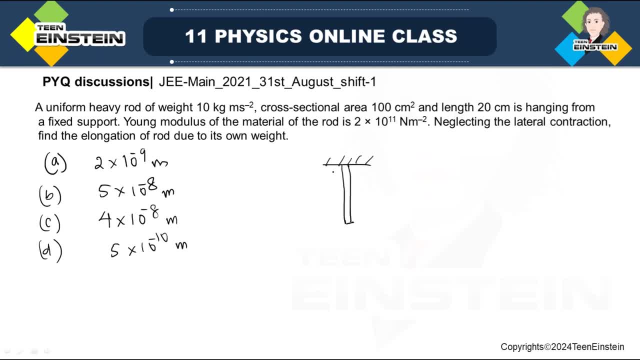 okay, i hope it is somewhat uniform. anyway, has got a length. okay, length 20 centimeter. okay, it has got length 20 centimeter. so it is very simple, right? we know young modulus is called stress by strength. it is the ratio of stress by strain, all right, so in this case stress will be white, weight of weight by area and strain will 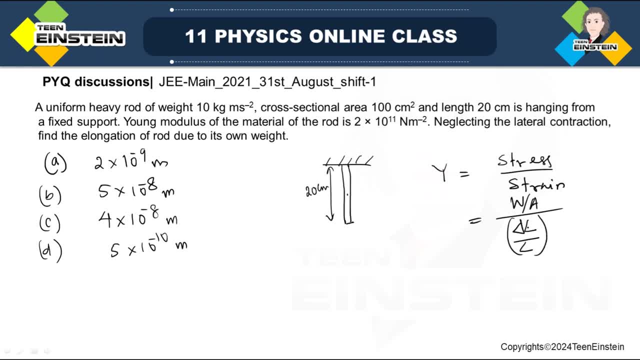 be suppose Delta L by L L is the original length, okay, and Delta L is the change in the length. so I have to find out what is the change in the change in the length. let me just do it see. I just want to find out what is change in the length. 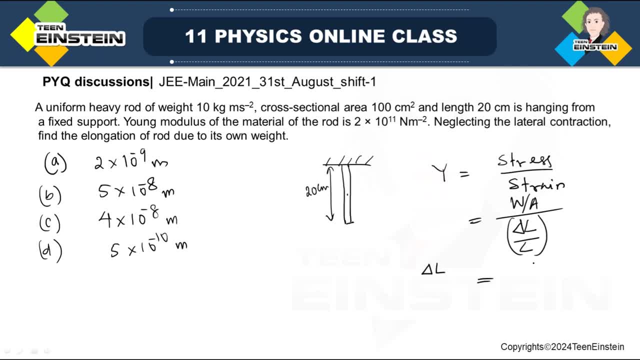 Delta L divided by W, by a, Y, a Y into okay, so Delta, L by L. so this L should go here. okay, W into L divided by Delta, sorry, a into Y. so this will be the change in the length, but in this case we one one just important concept you have to remember: in this case L should not, should not. 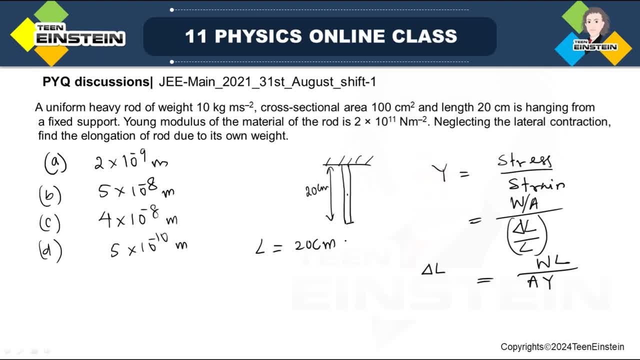 be taken as 20 centimeter. this is not 20 centimeter. it is 20 by 2 centimeter because we'll be considering the center of mass. okay, the point position of center of mass. from where the, or the center of gravity, since it is the uniform rod, the stress will be actually. 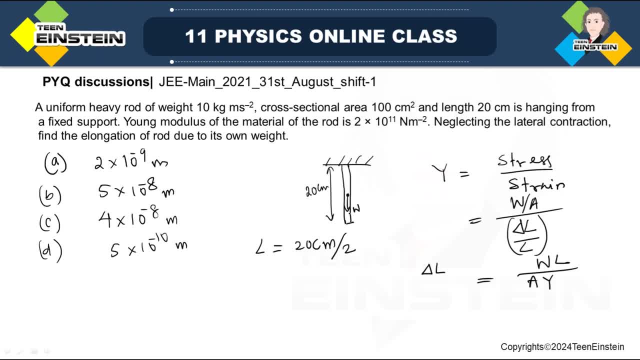 acting from here, okay. so where it will be? acting from here, from the center of mass, not from there, see, not from this end, okay. so that's why this length we have to consider as the original length, that is, L. L is then 20, see 10 centimeter, okay. so this is the important point you have to remember. 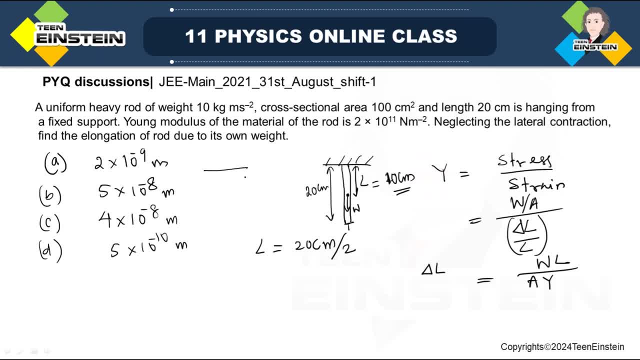 see this kind of problem even see- I'll just give you one more example- when there is a problem that a portion of chain is just hanging from a table, okay, table, so. so in that case also, you know the center of mass. see, if suppose the length L is hanging, the center of mass will be. 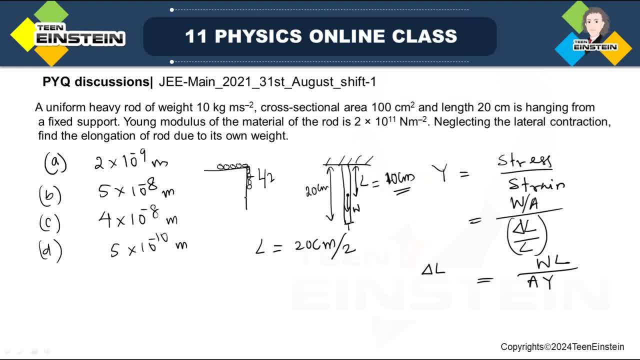 taken as L by 2 and in that way we have to consider the problem. so yeah, so I hope you remember this chain problem. all right, so similar to that is okay. so otherwise things are all right. so we will just write L by 2 over here. if I take the whole thing is L, then L by 2, or, if I have taken L is equal to 10. 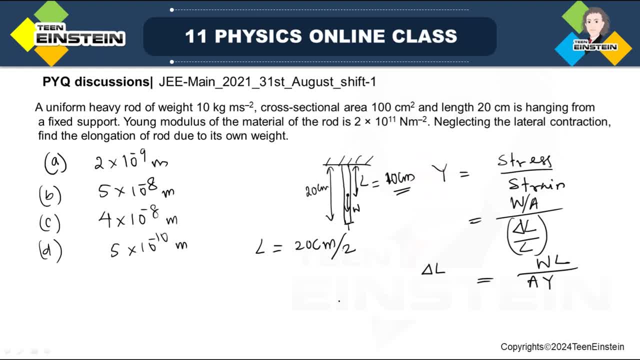 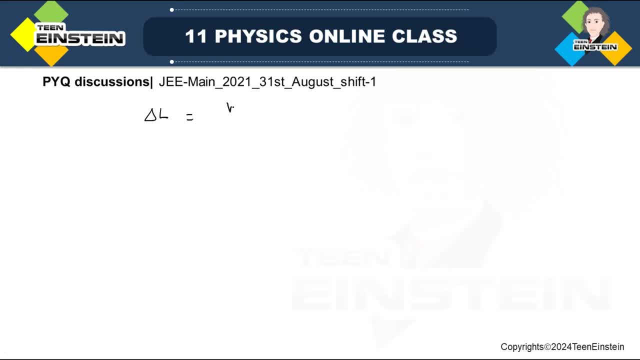 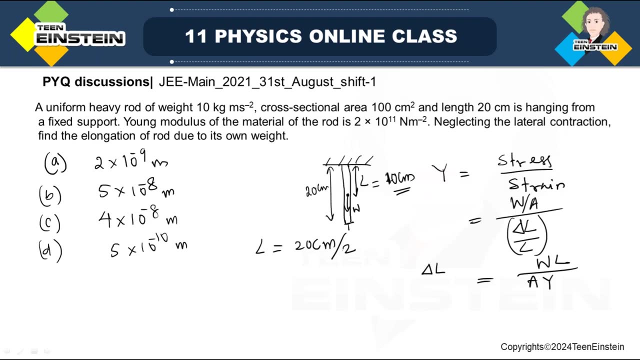 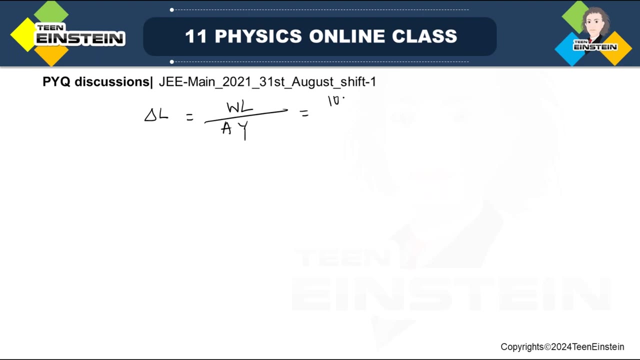 centimeter that soil. okay, so now we'll just put the values to get the answer. let me write it here: Delta L is equal to W into L divided by a Y. okay, so W the weight. or it is given as 10 kg. okay, so that is 10. 10 only see, l will be 10, but that is in centimeter. 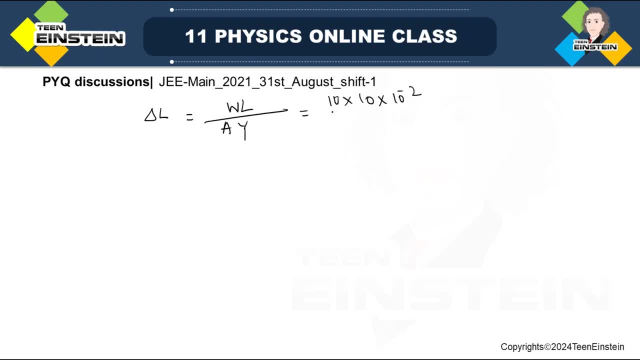 so i have to multiply 10 to the power minus 2. over here, divided by a, is the area of cross section that is given as 100 centimeter square. so i have to. i have to multiply 10 to the power minus 4 along with that to get meter square, and y is given as 2 into 10 to the power 11. newton. 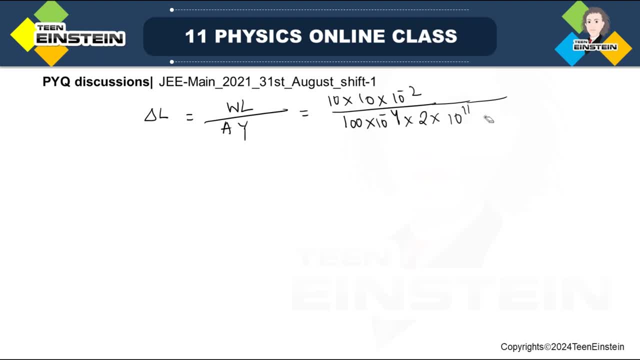 newton per meter square. okay, now it will actually give you in meter. okay, so let me see in which unit. okay, so eight, so there are all. okay, so let us do this calculation over here. so you have got see, these two will cancel each other. so you have here 10 to the power minus 2. okay, 10 to the power minus 2, so you will get 10 to the. 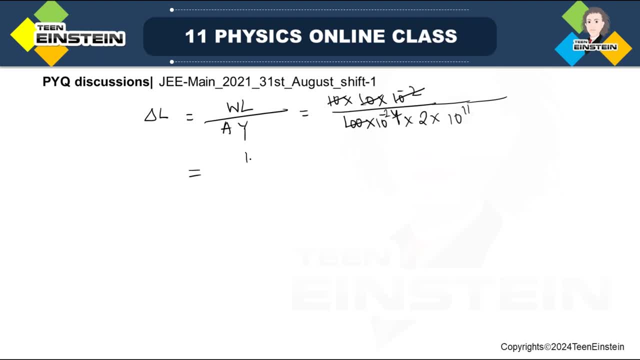 power 10 to the power 9 over here. so when it goes over, yeah, so 10 to the power 9 divided by 2, so it will be actually 5 into 10 to the power, it will be minus 9, so 5. oh, i see this will be 0.5, okay, 0.5. 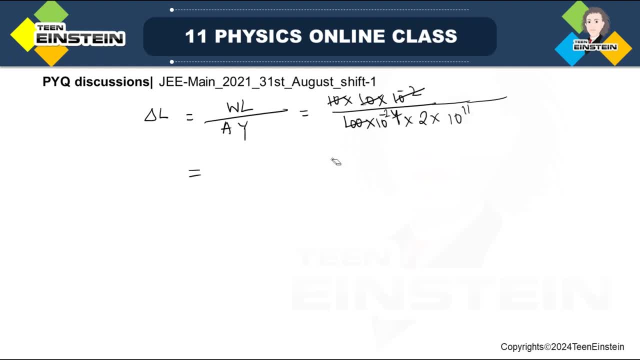 and just let me see once again: i have, i have 0.5. okay, 0.5 into 10 is bar 10 to the power minus 9. yes, so yeah, either we have to write 0.5 into the minus 9 meter. 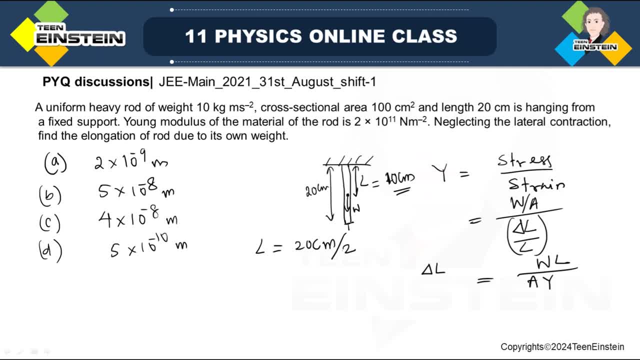 or we have to write 5 into 10 to the 10 meter. so what are the options given over here? okay, so it is. it is like this: 10 to the power, 5 into 10 to the power 8. let me just check whether you have done some mistake. okay, 100 centimeter, 10 kg, 20. yes, that's fine. 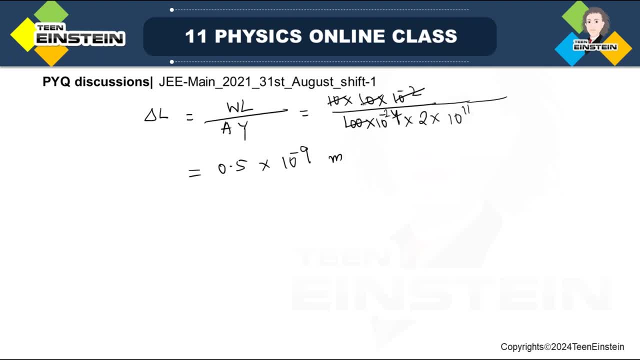 everything is fine over here. so this is yeah, 0.5. 0.5 means you know, 0.5 means 5 by 10, so it will be actually 10 to the power 9. over here it goes. i'm just doing a little mistake over here. 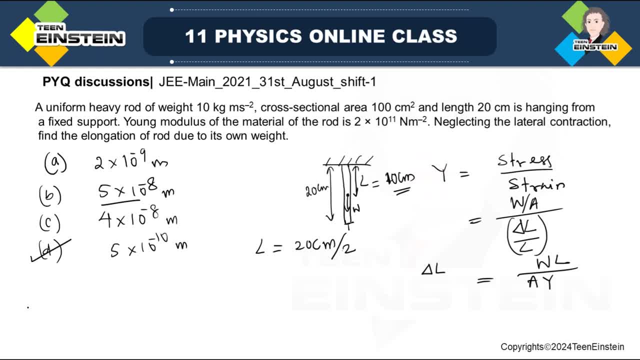 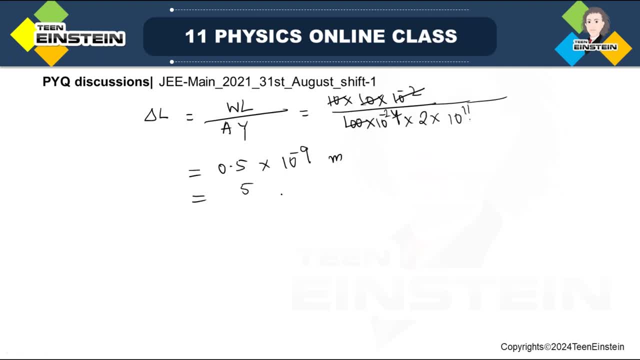 okay, i, i see i have options over here. see, i think i'm right. so it will be 5 into 10 to the power minus 10. yeah, so it is actually 5 into 24 minus 10.. yeah, i did not see the last option, so that's why i was in confusion. 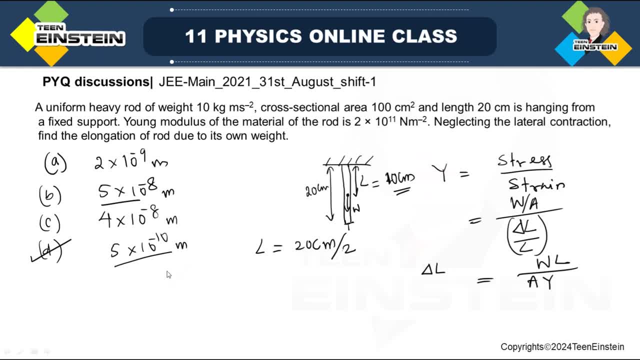 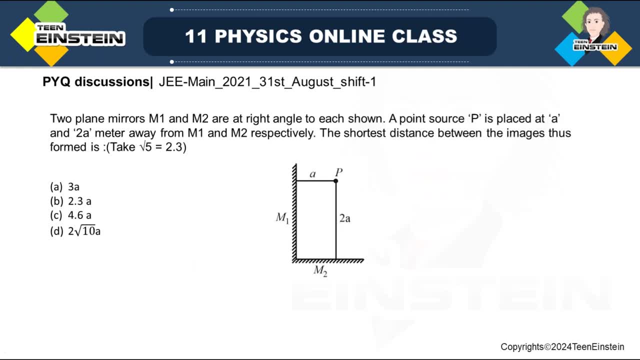 okay, so it is all right. so 5 into 10 to the power minus 10 meter is the answer. okay, so all right, we'll go to the next problem. okay, so this problem is really very interesting. this is from plane meter, so you see, these are actually suffix: m1, m2. okay, you can understand that. 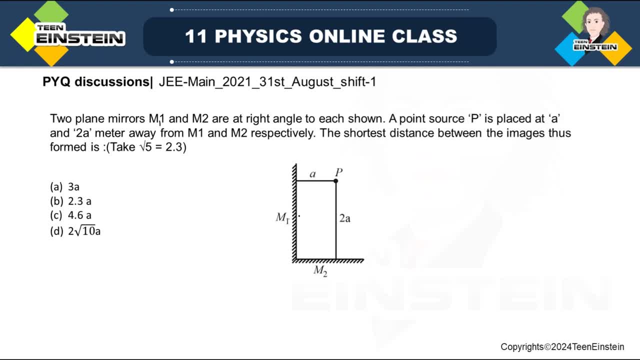 the plane meters m1 and m2 are at right angles. okay, these are two plane meters, they are at right angles to each other. a point p, a point source p is placed at a, at a distance, okay, a meter, a meter from m1, c from m1: a meter and two, a meter from m2 respectively. so the shortest. 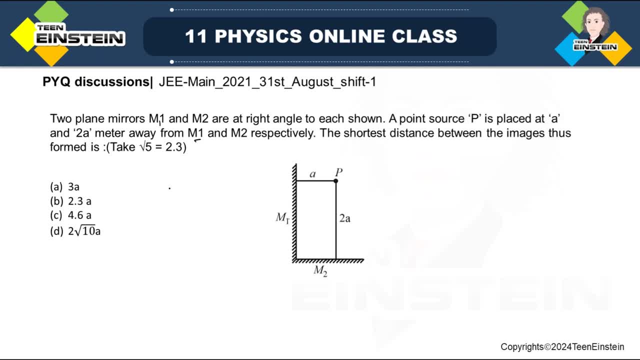 distance between the image is m1 and m2 respectively, so the shortest distance between the images thus form. look what will happen: there will be image formed here, somewhere at 2, 2a- okay, so here, 2a. distance away, somewhere here, 2a- okay, so for this, since it is plane meter at the same distance, it will be like: 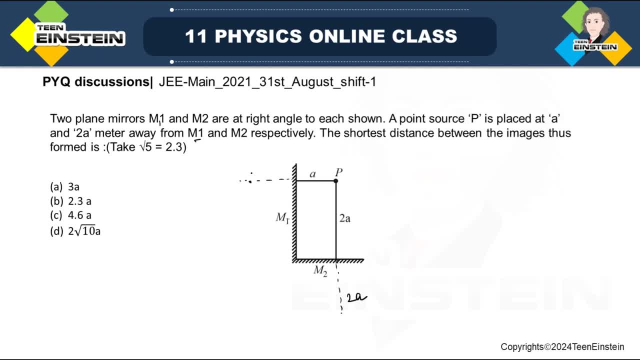 here somewhere. okay, so this is okay, so there will be one, so there will be one image over here. let us say this is image over here. let us say this is image over here. let us say this is i1 and this is i2 okay, i1 and this is i2 okay. 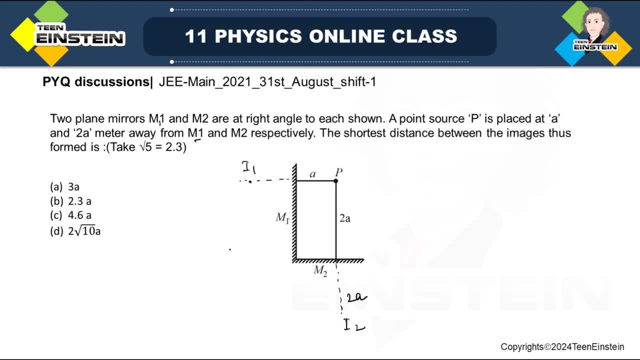 i1 and this is i2. okay, so generally. if we consider this to image itself so generally, if we consider this to image itself so generally, if we consider this to image itself, look, this distance is actually this is 2a. look, this distance is actually, this is 2a. 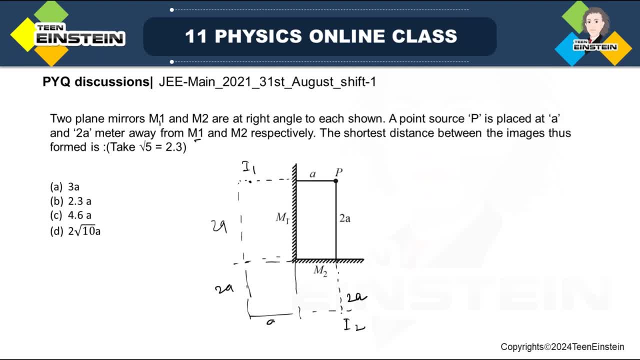 look, this distance is actually. this is 2a, this is 2a- 4a, and this is this is a. this is a 2a okay. this is 2a- 4a, and this is this is a. this is a 2a okay. 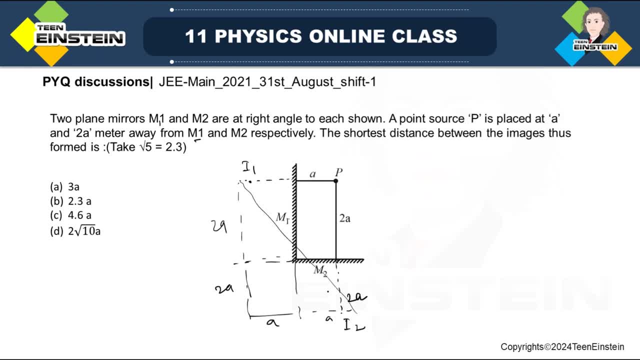 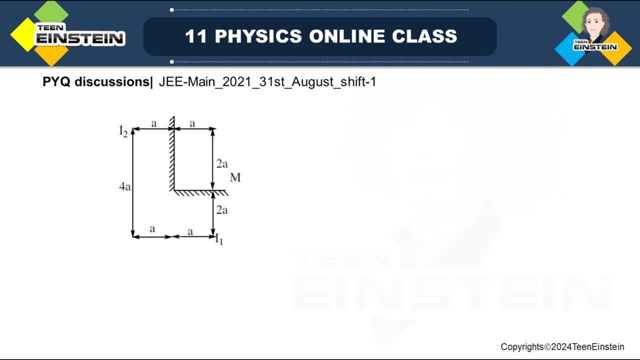 this is 2a, 4a and this is: this is a. this is a 2a. okay, so i have to find out the distance between them. so that means this one. okay, let me show you the proper figure over here. so see, we need to actually find out the distance between these two actually. 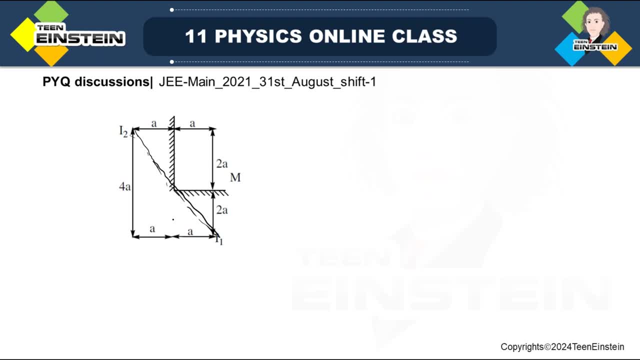 this hypotenuse of this right angle triangle. so you know, we have to find out this hypotenuse. so this distance is square root of 4 a square plus 2 a square. okay, so you'll get 16 a square plus 4 a square. so that means, uh, 20 square, so a into 20. i can do one thing. i can just. 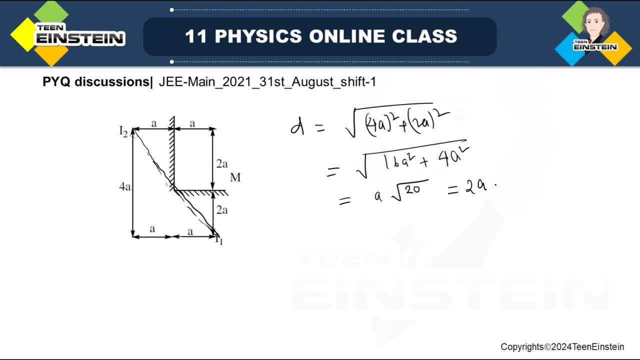 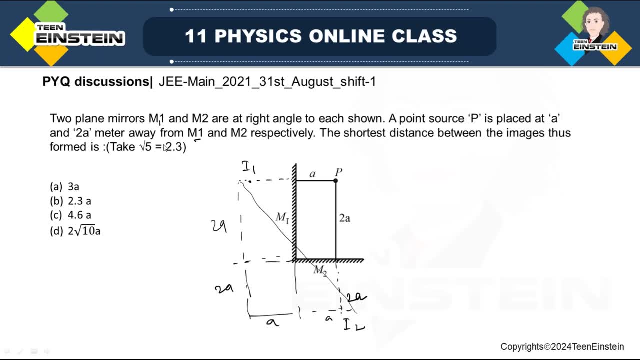 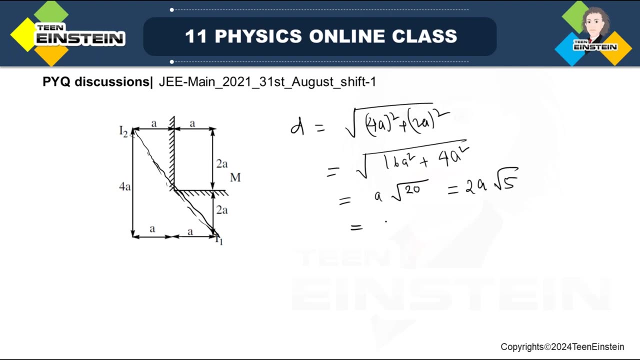 write a 2, a root over 5.. so there is actually given to this 0.5. sorry, square root of 5 is 2.3. square root of 5 is 2.3. so if that is the case, look 2 into a, into 2.3. so it is. 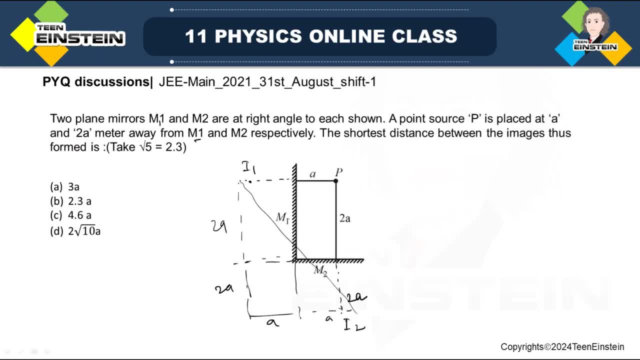 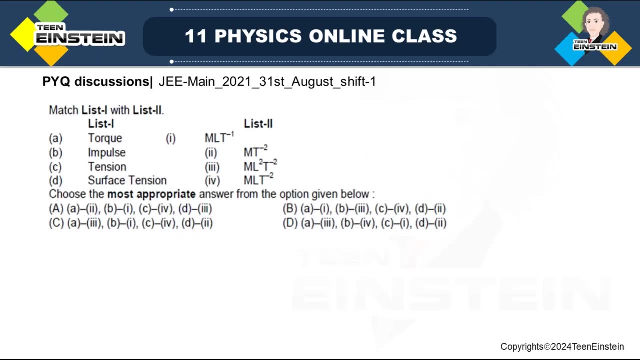 4.6 a. okay, 4.6 a, and see there is an option over here, so option c will be the correct answer for this question. okay, so this is done. let us go to the next problem. okay, so this problem. see, there are two lists, list one and list two. we have to match the dimensions with the quantities. 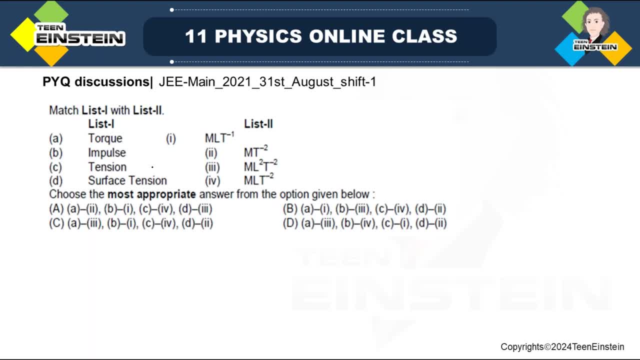 okay, we have to match the dimensions of the quantities given in the list of one with the uh dimensional formula in the list two. okay, so torque. let me write one by one. so see a. okay, let me just do the torque over here. torque is actually r? f sine theta. sine theta is dimensionless quantity. 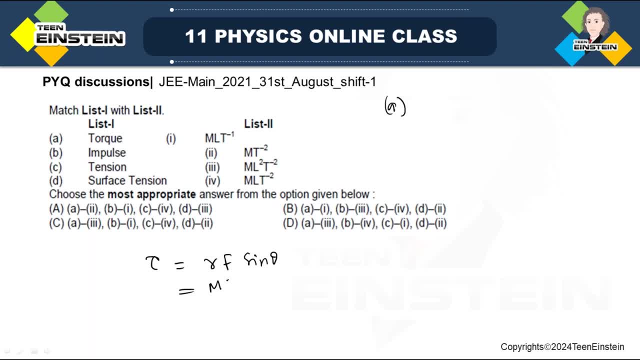 this is f and r. okay, so this is m l. this is m l t to the power minus 2. that is the force and this is l. so i will get m l square t to the power minus 2. in fact, this has unit of energy, or one ton. okay, m? l squared minus two. so this three. so a will match with three. 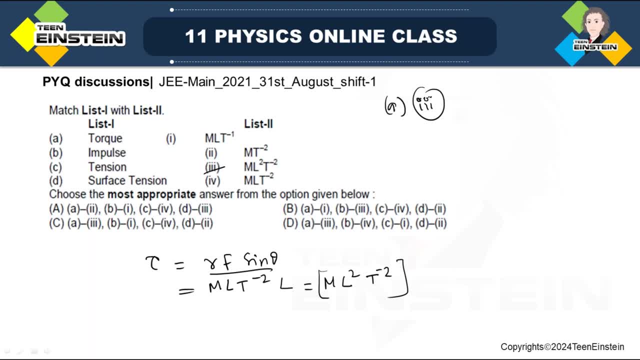 okay, a will match with three. all right now let us go for the impulse. you know impulse is actually f, period, ah, f flow with a coordinate direction. okay, a is equal to r. encouraged b is brunch lobby. the impulse is denoted by i or j. let me denote that with j. 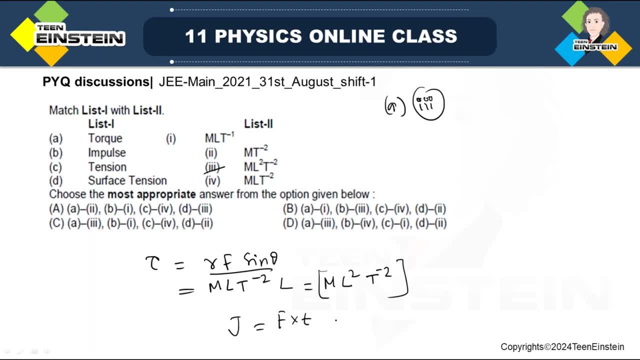 impulse is f FIRST into t force, into time, time. it is divided down to infinite impulses. impulse is denoted by i or j. let me denote that with j, let me know that with j. so j is actually f into t force, into post time force, entire. so we know m? l? 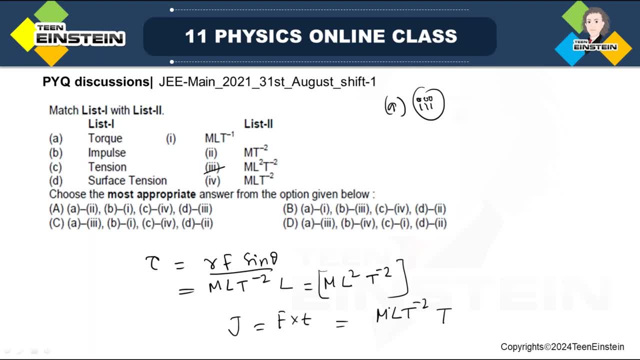 impulse is denoted by i or j. let me denote that with j, so j is actually s into force, into force, into time, so we into t. okay, so your ultimately dimensional formula will be will be m? l to the power minus one. let us see: m? l to the power minus one, so one. 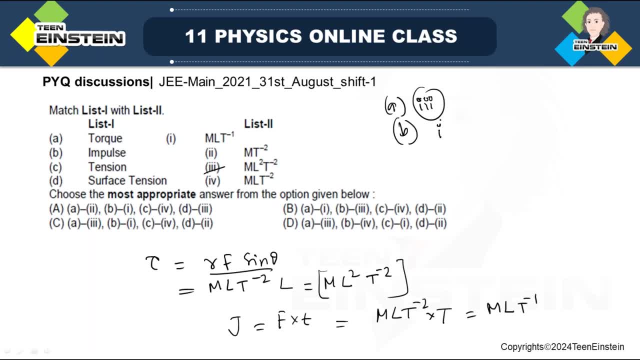 so b will actually match with one, all right. so let me clean this portion again, so so that we can do the other one. okay, tension, tension is simply force. right, tension is simply force. okay, tension is simply force. that is m l to the power minus two. so this: 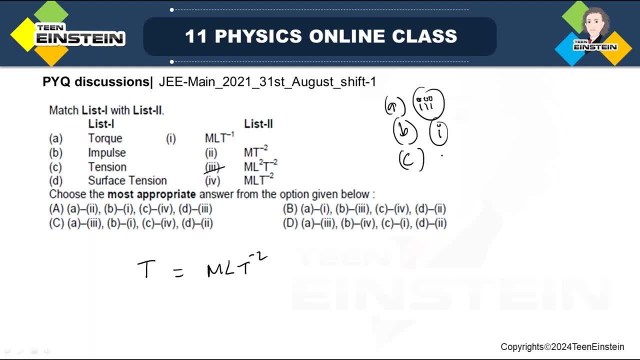 will be four. so option c will match with four. let us see the d. surface tension is actually f by l. f by l is equal to surface tension. okay, let us denote that by s. okay, surface tension is f by l. f by l means m to the power minus two, so it is actually matching with two. so it will be m- t to. 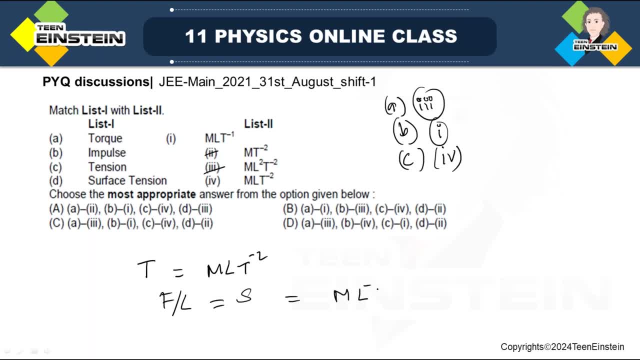 the power: m to the power minus two. l will not be there. m to the power minus two. okay, so d will be equal, so t. okay, so this is so a3. let us check a3, b. no, this is not the one. a3, b1, c4, d2. okay, so option. 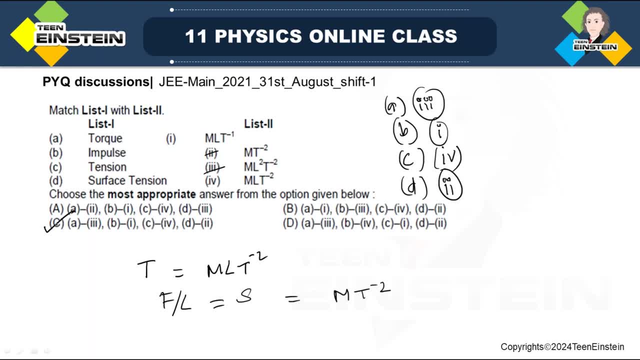 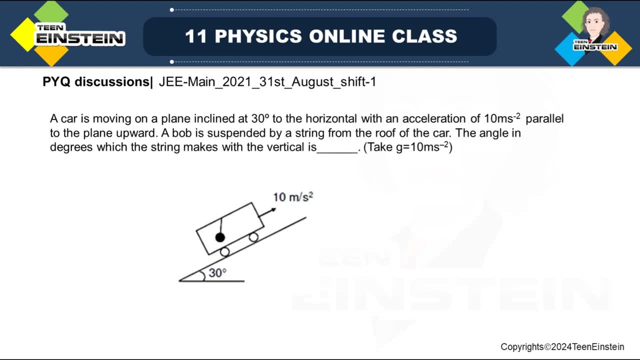 c will be the correct answer for this question. all right, so let us go to the next problem. okay, so this is a very, very important problem we have to solve here. a car is moving in a plane incline at 30 degree to the horizontal, with an acceleration of 10 meter per second square. 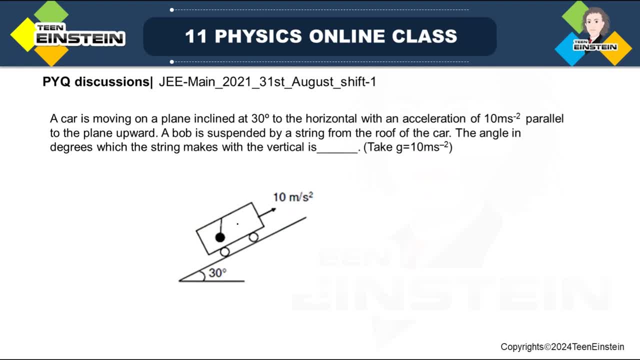 see, this is a car. you can see that a car is moving upwards. okay, this is parallel to the plane upward. okay, car is moving in a plane, inclined along this inclined plane in the upward direction with an acceleration. this is a, so this acceleration is 10 meter per second square and inclination of this plane is 30 degree, with. 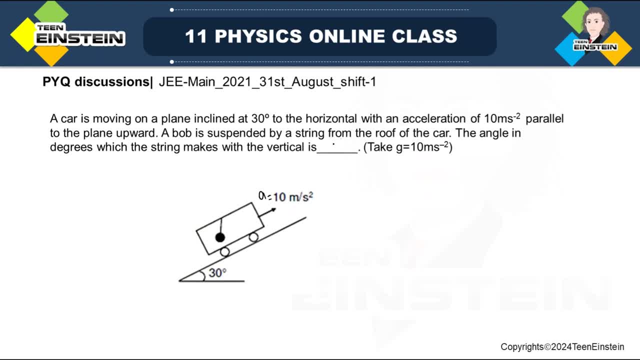 the horizontal. this is given a bob is suspended by string from the roof of the car. you can see that this is the bob which is suspended from the roof of the car. the angle in degrees which the string makes with the vertical, with the vertical, is this: okay, you have to find out that, actually, okay. 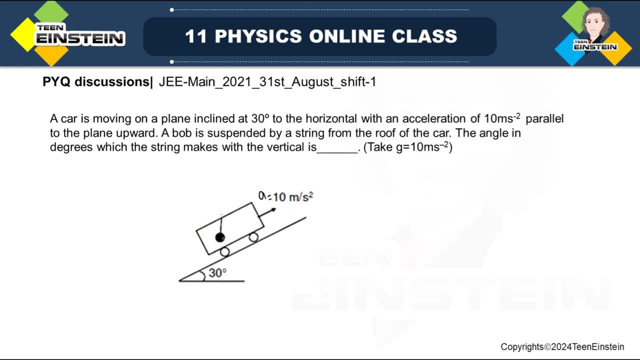 so, while it moves, see, you know, see you have here, see, in inclined plane, first of all, the g will actually act vertically downward, like this, okay, but it will actually makes an angle: 30 over here, okay, 30 over here. so this is actually mg, boss of theta, that you know, all right, and amg sine theta, which will act. 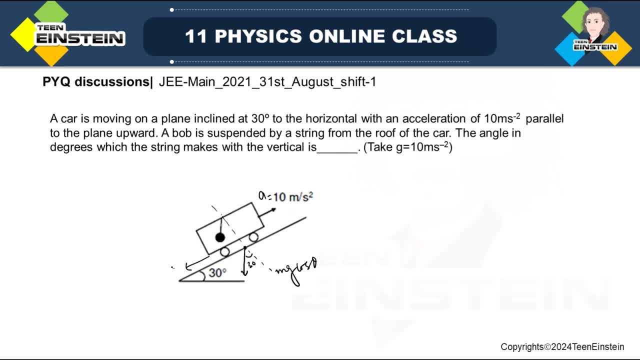 this way. okay, so amg, if the mass of this car is m, so amg, sine theta will act in this way. all right now for the bob here. for the bob: see, it is already in the inclined plane. see, see, mass should have gone like this. so this angle is not only theta, actually, see, i would have drawn here. let me draw the figure over. 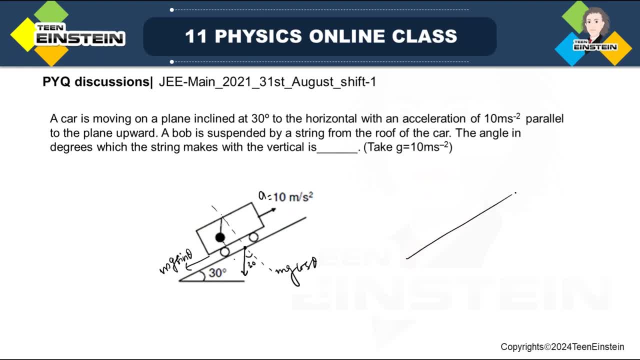 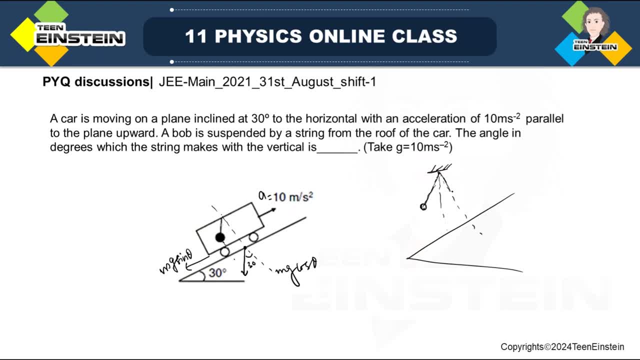 okay, and this is, this is the perpendicular to the plane. okay, and this is actual vertical vertical to the ground. you can say: this is the, this is the actual vertical to the ground. okay, now, this angle is theta. i know, 30 degree. sorry, this angle is 30 degree. 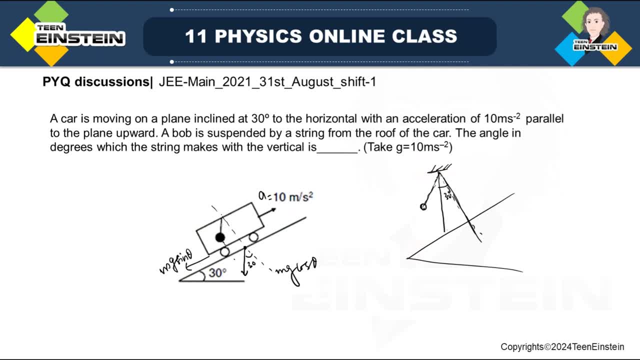 zero. you are far from zero. there you go. i know this triangle exactly. Signes are like that, so let us draw safety. okay, now i want you to imagine somehow that you are. i want to draw a reference here. so this one we are watching improves three phi. 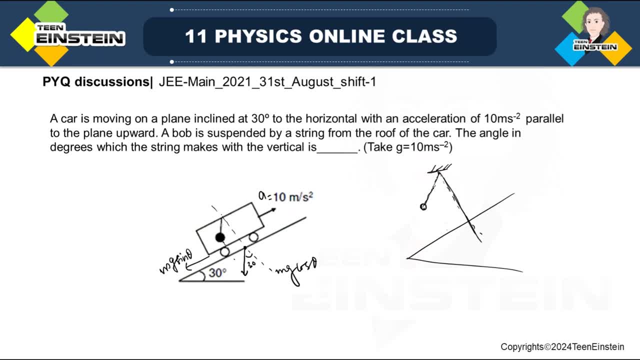 and k equals zero. you want to learn that? okay, now you want me to explain you你要 let us take this angle. so what is this angle actually? this angle is the particle actually. this is the particle with this, this car itself. okay, in this car, this is: 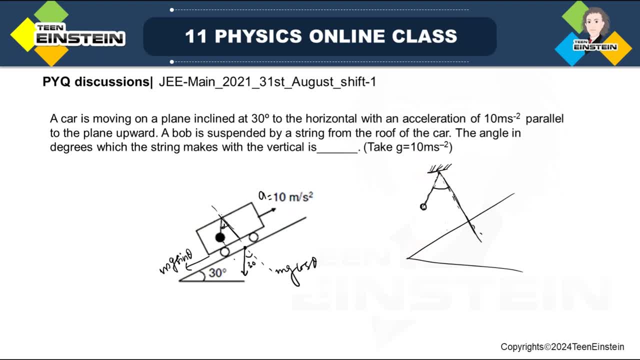 actually the particle right. this is the vertical, so I can take this as this actually. so this angle is actually not see. the original particle will be like this, like this, as I had drawn earlier, but we have to actually I'm sorry, so let me just draw it once again. okay, this is, this is 30 degree, so you know this will. 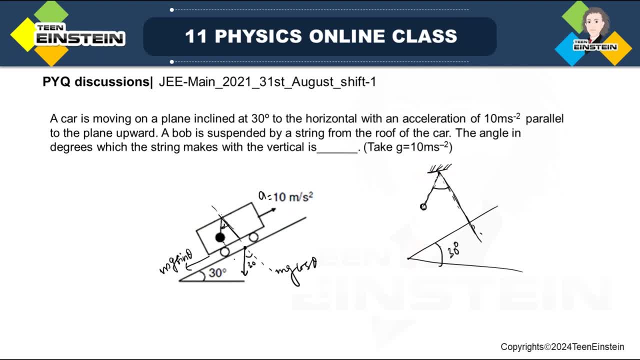 be. actually see, your G will be like this, G will be like this, so this angle will be 30 degree. so you look, if this, yeah, so if this is the, this is particle, it is actually particle to this. suppose this is the particle one. okay, so this is 30 degree. we know already, this angle is 30. 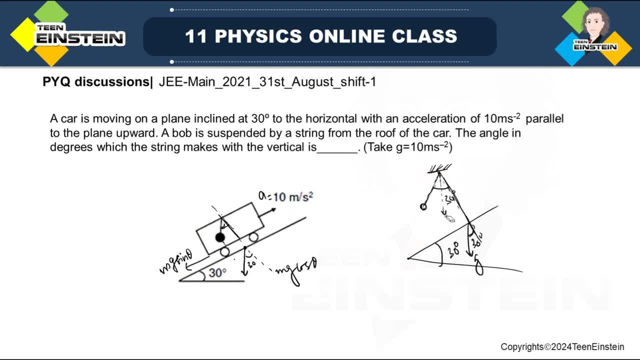 degree, but we have to find out the angle, this angle, this much, okay, so I'm sorry. this look, this angle is 30 degree. let me draw it properly. and this is some Peter say. I hope you have understood now. this is the Bob in the car which is here. you can see that, okay, so you just go just. 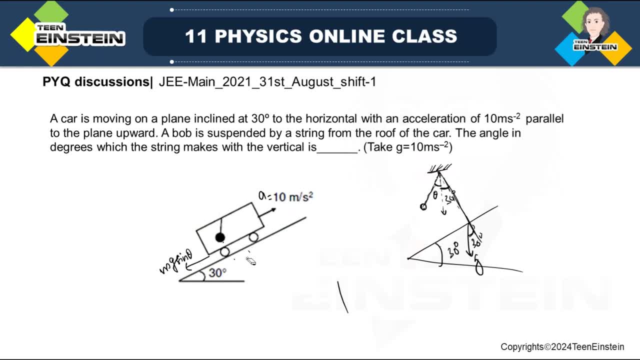 don't get confused with this. you got a diagram. let me show you here. this is the situation. okay. so you look here: G will be acting like this. so G cos theta. this is G Cos theta, okay, which will actually be like: okay. so this is generally in general. if there is a block, n will be acting like this: G cos theta, okay, okay. so if that is a block, and will be a. 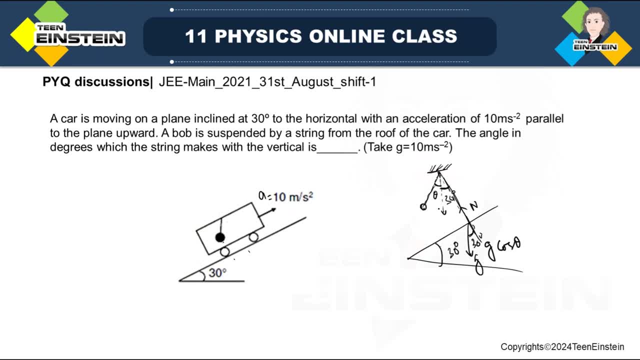 in this way. okay, that that is what we knew. okay, now the situation is: see, we have to find out the angle angle with this vertical, because, see, the vertical is like this. now, okay, we have to find with this angle. okay, original vertical is this one and with this vertical, this angle is actually 30. 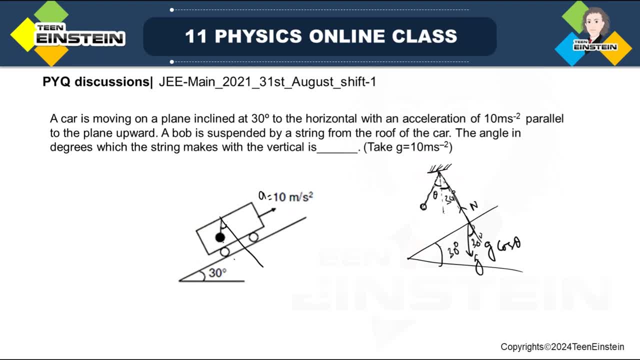 degree. okay, but we have to find out the angle with the vertical to this support. okay, this supporting with respect to this support, it is the vertical. okay, that is perpendicular to the inclined plane. so that is the vertical here. so this angle obviously is 30 plus something, some theta. i hope i am able to make you understand. this is the situation here, right? 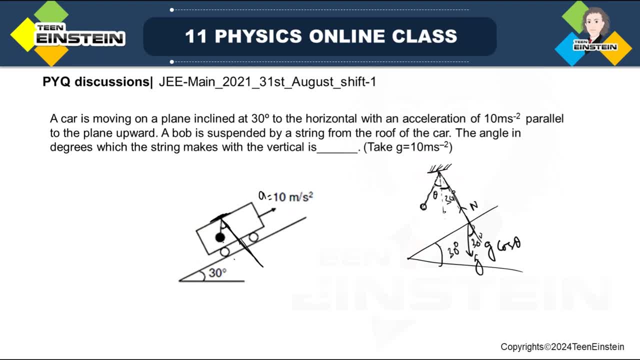 okay, so with this i have to check. so here, look what happens with the bob. what are the forces acting with the bob? see, there are. see, if i just consider the tension, so tension will be acting like this, so it will be like this, okay, i mean, see, it will be actually. 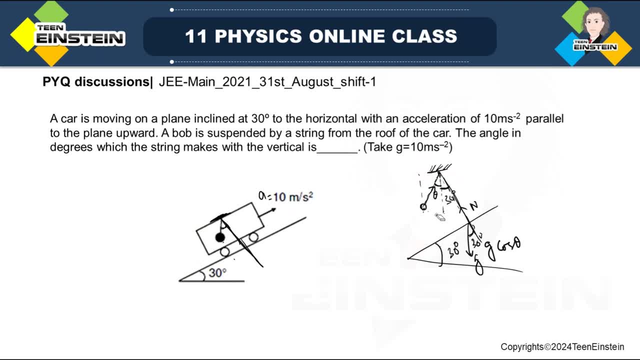 so everything is right. that means hanging something. so if it is bad, all right. so the tension will be like this: carefully, now, you will not interested. the tension will be acting like this: okay, and as i have already said, so if the tension, If this is theta, this is also theta. So T cos theta, and this way it is actually T sin theta. Now look, with this inclined plane, what we have along this direction, So at the equilibrium position, this angle is theta. 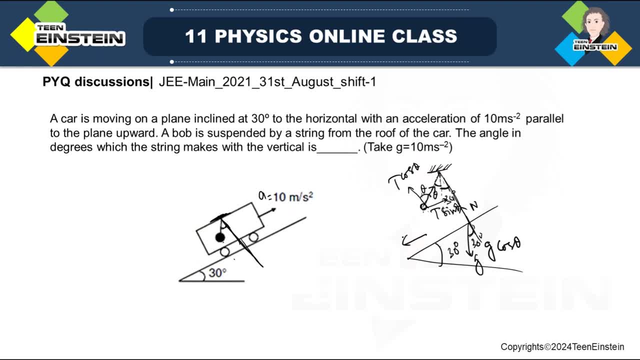 Okay, so at equilibrium position, see on the inclined plane, if I just take, the whole system has mass M. in that case, you know, you will have Mg sin theta in this direction And since it is moving- see on the bob- there will be another pseudo force, since it is moving in this direction with Ma. So there will be a pseudo force acting in this way. 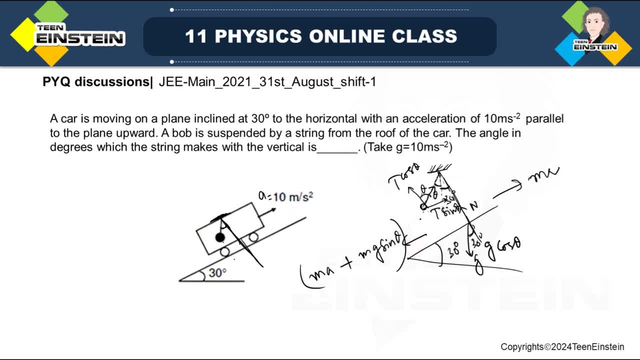 Okay On the on the bob. Okay On the bob. there will be a pseudo force acting this way. So I can actually consider the equilibrium situation when Ma plus Mg, sin of- sorry, this is not theta, this is 30.. 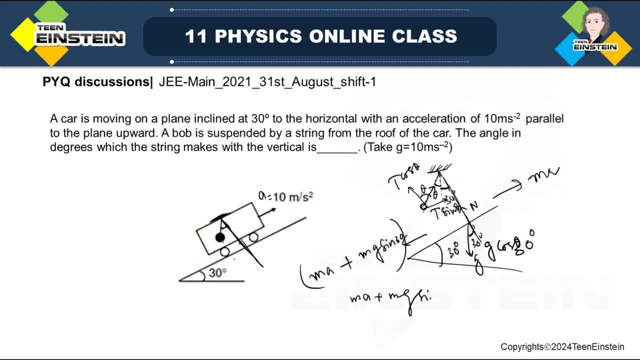 This is 30.. This is 30 degree. Mg sin 30 degree will be equal to the 10th, and see this sign. theta component T sin. theta plus 30 degree. theta plus 30 degree. Okay, so I think this is this way, okay. theta plus 30 degree. 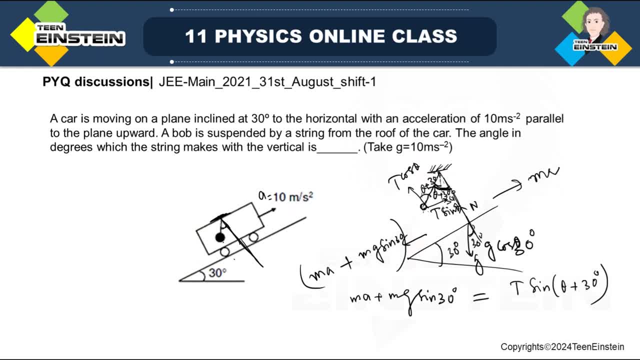 This is the whole thing, Okay, theta plus 30 degree. Okay, let me plane it. It has become too much messy. Okay, so see, this angle is 30.. this one and this is theta. okay, so this will be total 30 plus theta. 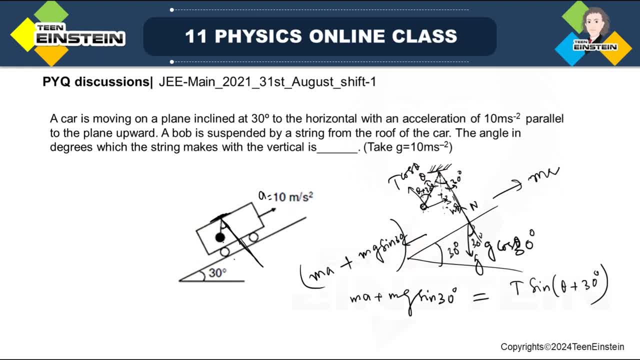 the whole angle. so this will be okay, all right. so tension acting in this way. so this will be t? sine of 30 plus theta, okay, 30 plus theta along the inclined plane, and this way it will be cos of 30 plus theta, okay, and in the vertical direction. 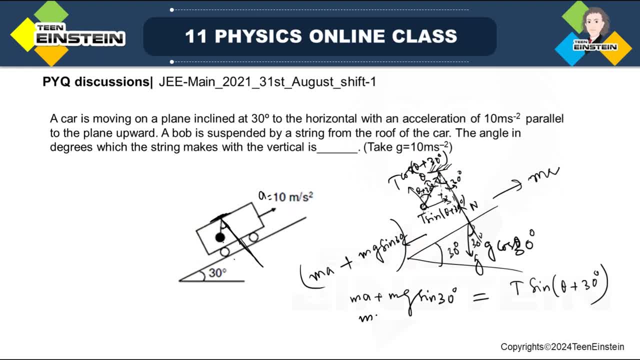 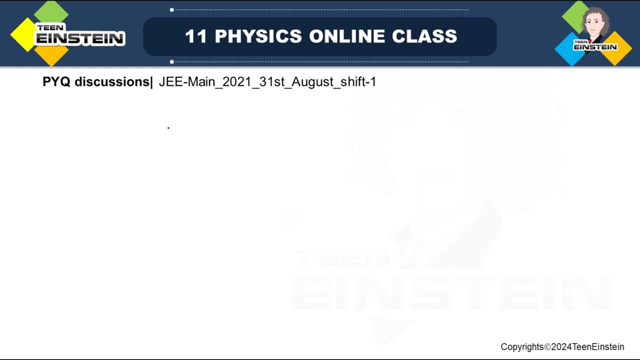 see vertical direction it will be: mg cos of 30 is equal to t was of 30 plus theta. okay, so this is the free body diagram over here. okay, so if i take the ratio of this two, what i'll get? i'll just write in the other page. see, i have t. 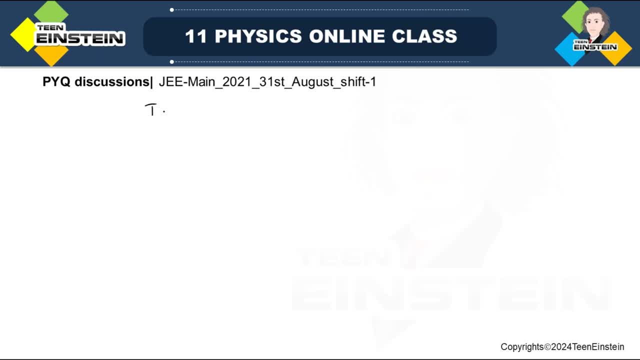 okay, t sine of theta plus 30 degree, which is is equal to m. g sine of 30 degree plus pseudo force in the bob, that is m, into a. okay, here t cos of theta plus 30 degree. along with that, there will be okay, so mg cos. 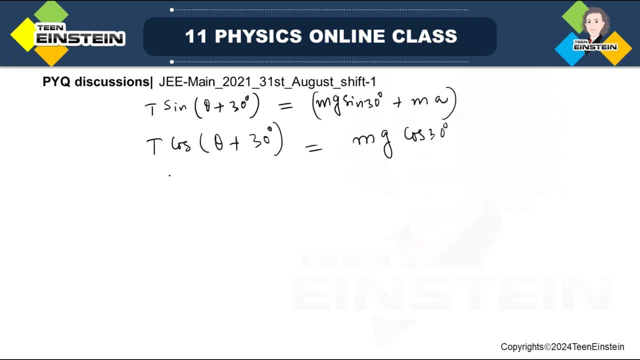 of 30.. all right, so here if i take see, just divide these two, then i'll get. i'll get 10 of 30 plus theta degree is equal to see m g into half plus m into a divided by. so this is pos 30 degree. that means root 3 by 2, root 3 m g by 2 over here. 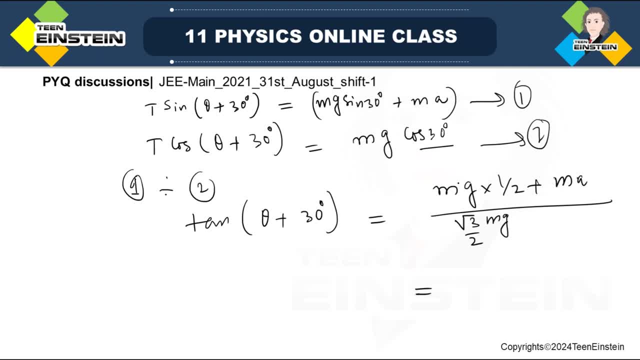 so i'll just get this c, m, i don't know i can actually cancel from both sides like uh, from the denominator and numerator. so then the g is 10, so 5, plus this a is 10, so this I have got so 2 into this divided by root over 3. okay, so 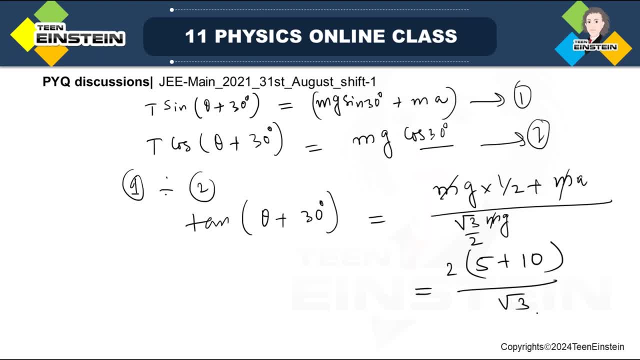 this will be actually 30, and see this G also is there. so this is 10, so you will get see 30. that was 3 by root 3, 3 by root 3. that means 10 of 30 plus 30 degree, which is is equal to root over 3, and we know 10, 10, 60 degree will be. 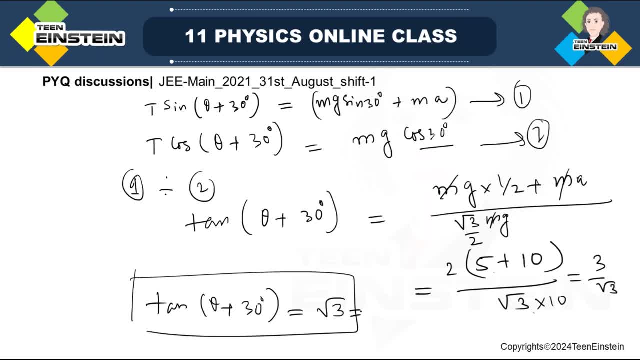 equal to root over 3, so this is actually equal to root over 60 degree. sorry, 10, 60 degree. okay, now this and this argument we can equate. so from there we'll get: theta plus 30 degree is equal to 60 degree, and that is giving you theta is equal to 30. 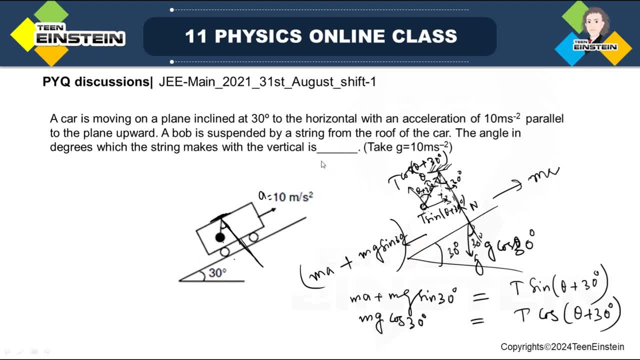 degree. so here this angle will be 30 degree with the particle. okay, so 30 degree will be with the particle. okay, so theta will be actually 30 degree. all right, so with the particle it will be actually theta, so that is 30 degree. I hope you are understanding this situation over here. all right, so we'll go. 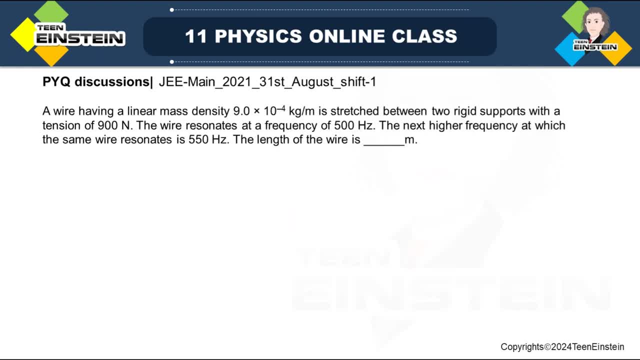 to the next problem. so this problem is says, in saying that here we're having linear mass density, linear mass density 9 into 10 to the power, minus 4 kg per meter. okay, that means mu is given for a strain. okay, this is kg per meter. is stress between two rigid support? that means this one. 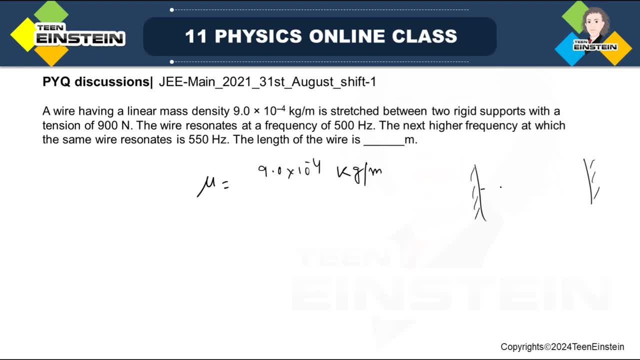 this is actually a problem from straight stream with the support and the tension of the support is like a string in the string is 900 newton. the wire resonates a at a frequency, at a frequency, 500 hertz. the next higher frequency at which the same wire resonates is five. 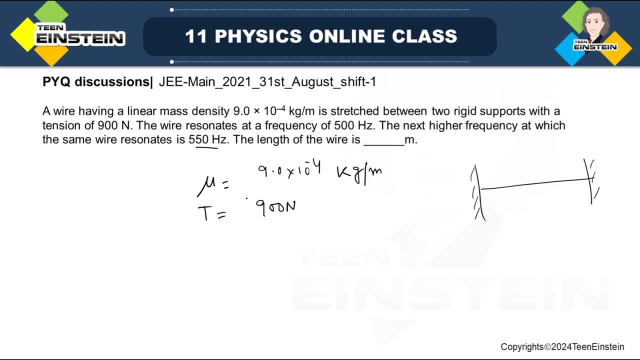 50 hertz. so i have to actually know or recall here what is the formula for the harmonics or what are the harmonics generate in the straight string. so we know this will be actually: mu is equal to p. v by 2, l, and you know this is actually. p is actually one, two, three, four, five, all even and 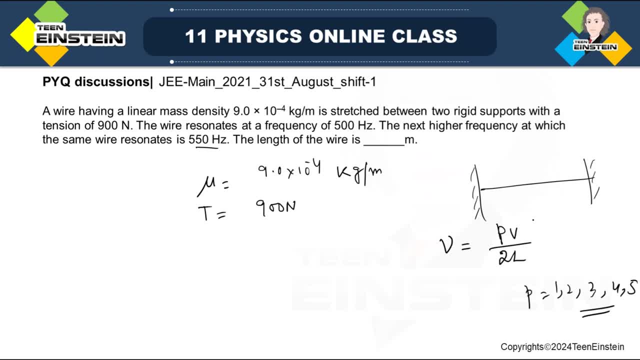 odd harmonics are actually created in stage three. now here, according to this problem, see new: p is 500 here, this is v, this is the velocity. so this is the velocity of some, like a wave, stationary wave in the string of wave, in the stream or through the string. 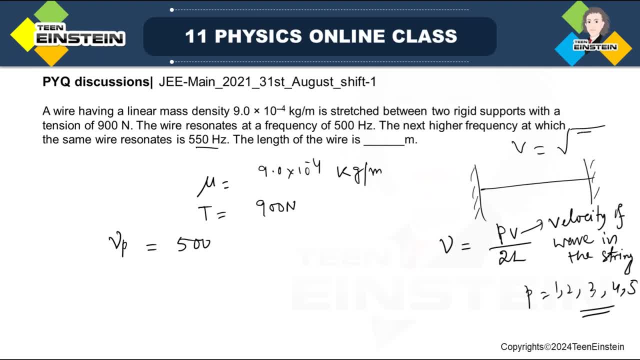 and that has got a formula: v is equal to root over t by mu. this we can find out anyway. so this is given as this one's hertz and nu, just next one new p plus one that is 550 hertz. okay, all right. so here, if i just 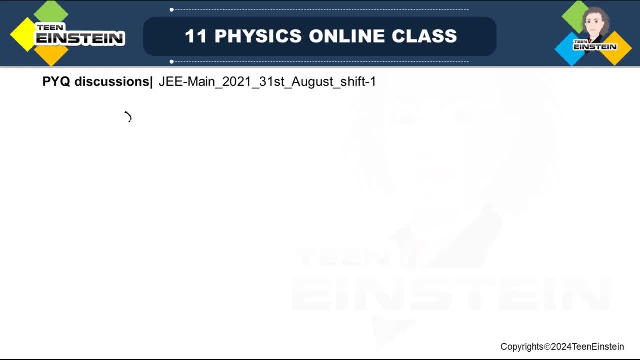 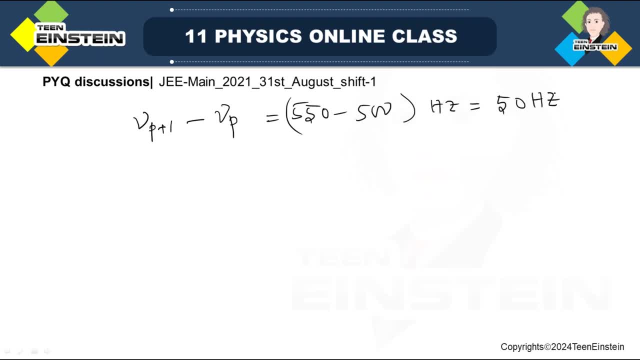 that gives you 50 hertz. okay, now this: I can write p plus one into v divided by 12, and this is p, v by 2 hold, which is 50 hertz, okay, so see, if I just take this, okay, So P will cancel each other, So we'll get actually: V by 2L is equal to 50. Right, So I have to find out the length of the string over here. Okay, We had to find out the length of the string in meter, Okay. 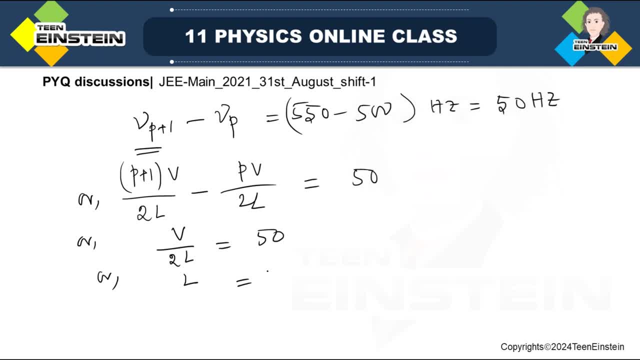 Okay, So L will be V by 100.. So what is V? V is square root of T by mu by 100.. So what is this T? T is given as 900 Newton tensile, And this is 9 into 10 to the power minus 4 divided by 100.. 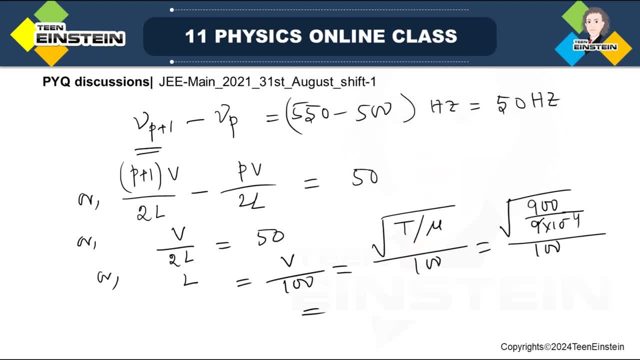 So this will actually give. you see, this will Cancel. So this will be 10 to the power 6.. Square root of 10 to the power 6 will be 10 to the power 3. So I'll get 1000 by 100. That means it is 10.. 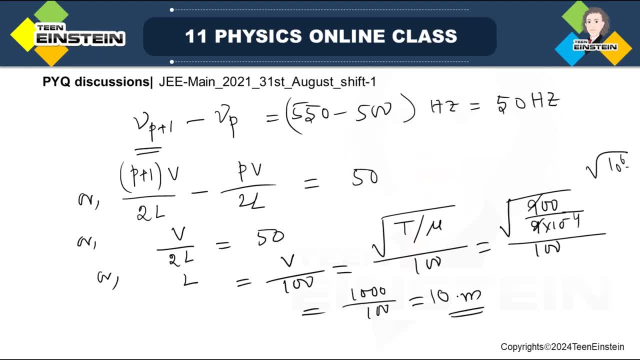 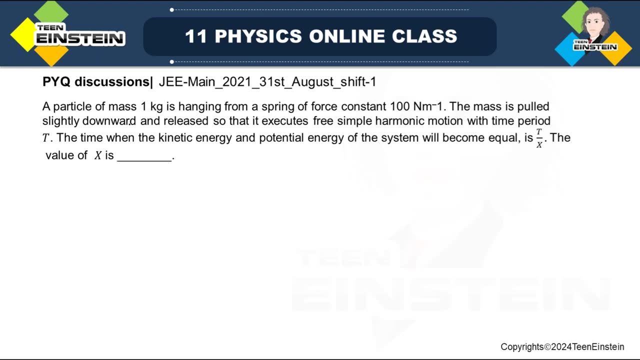 So length of the string will be 10 meter. Okay, So this is 10 meter. All right, So let us go to the next problem. So this problem is also very, very interesting. A particle of mass 1 kg is hanging from spring of force constant 100 Newton per meter. 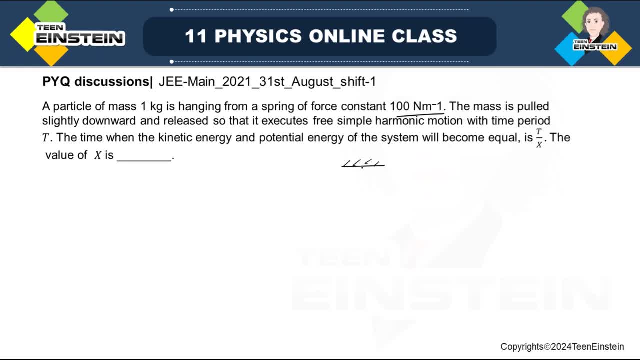 Let me tell you this: So there is a spring, So it is hanging, Okay, So there is a mass attached to it. Okay, It is just pulled. It is pulled and leaped. Okay, So it was pulled and released. 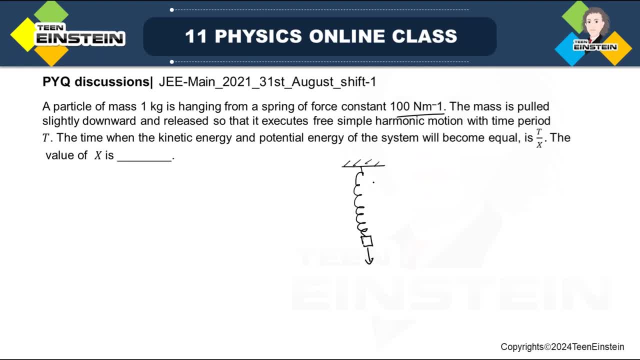 So that it executes simple harmonic motion. As you know, it will execute simple harmonic motion. if you pull it and release, Okay, What will happen? What will be the result? The result will be SHM- Simple harmonic motion- will be there in the spring. 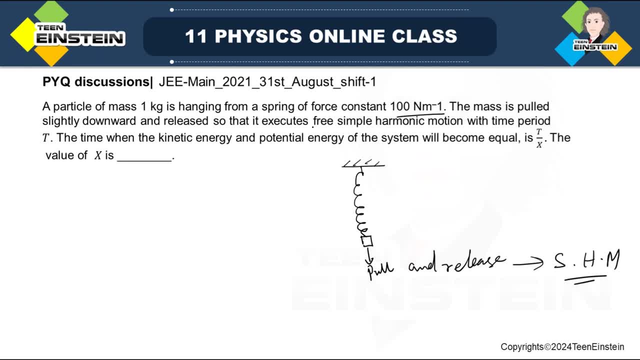 Okay, So the question says it executes free, simple, harmonic motion with time period T and time period of this motion will be T. The time taken- Sorry, The time when the kinetic energy and potential energy Of the system will become equal is T by X. 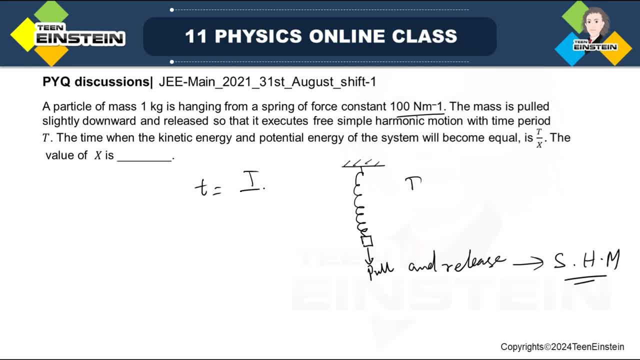 That means T small t is equal to T by X. this time, the kinetic energy and the potential energy of this spring, which is oscillating in simple harmonic motion, will be equal. Okay, kinetic energy and potential energy will be equal. So what is this? X? 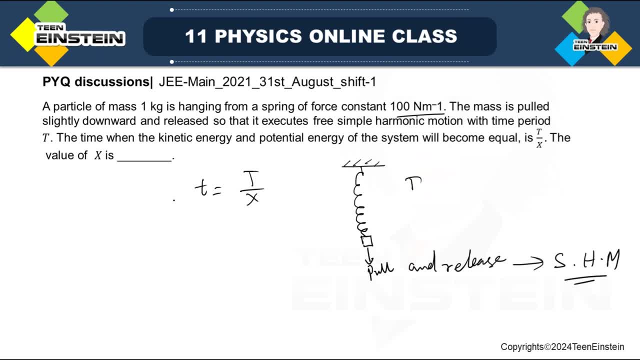 So what is this X? So what is this X? So, look, this question is very, very simple question. I know, Let me find. let me just take the displacement For SHM. you know, displacement will be a sign of omega T. 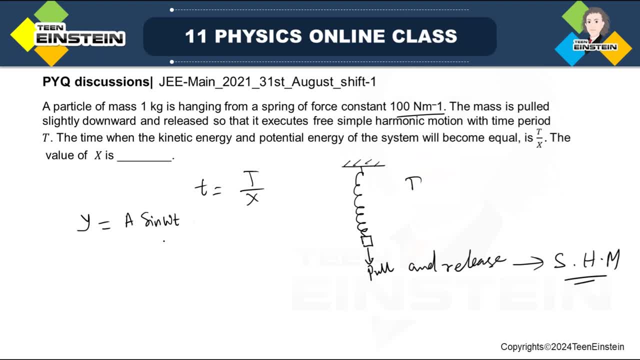 I'm just writing phase initial phase to be zero. Okay, Like this. Now let me find out what is kinetic energy. So what will be kinetic energy and what will be potential energy? Let me find out. So let me take at this particular displacement, arbitrary displacement- the kinetic energy will be half MV square. 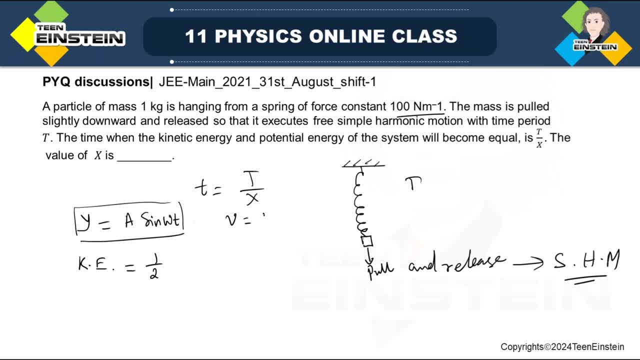 Okay, What is V in case of simple harmonic motion? We know that it will be a into one minus Y, square by displacement, square by amplitude, square Y, square by a square Right, I'll just move that. So this is velocity at any displacement Y, arbitrary displacement Y at time T. 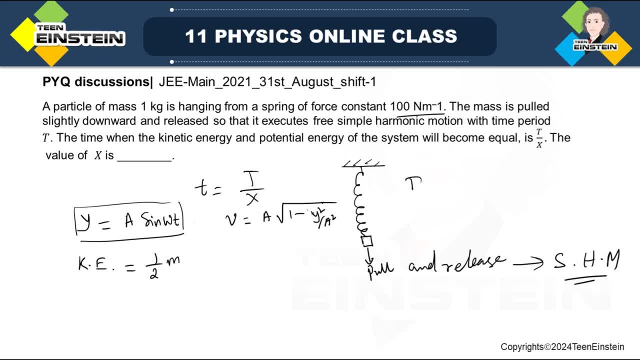 So half M. let us take this. M is equal to one KZ. Okay, So let us take that as M itself. here, M half M V square, That is half, That is half M. CV means this is a square. Hold it to one minus Y square by a square. 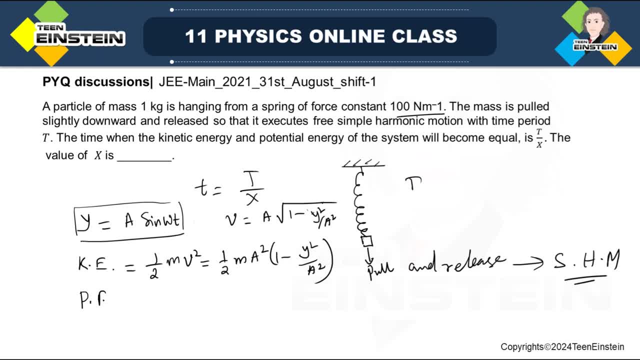 Let us keep like this. What is the potential at this particular displacement? That will be half K Y square. Why is the displacement right? Okay, So K is the K is actually. See, it will be omega square into M. okay, omega square into M. 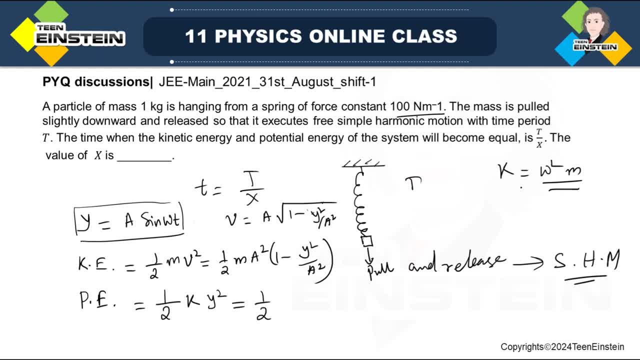 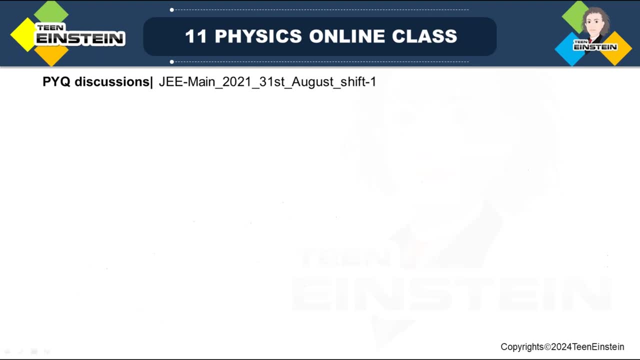 So let me write that, because we know K by M is called omega square for simple harmonic motion. So half M omega square, Y square And according to the problem at this particular time. Okay, So at this particular displacement, potential energy is equal to kinetic energy. 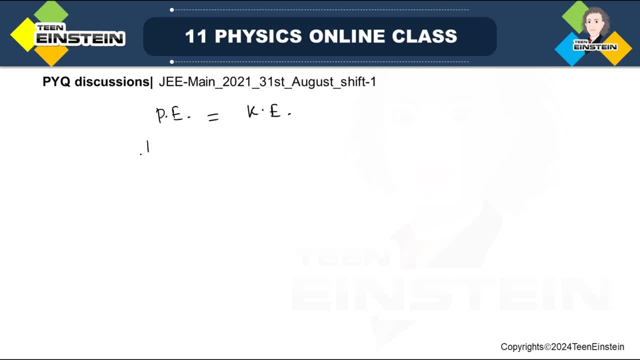 So I can write half M omega square. Y square is equal to half M A square omega square. I think there will be omega over here. Okay. Okay, Let me write that. Yes, So this is the potential energy I can write. 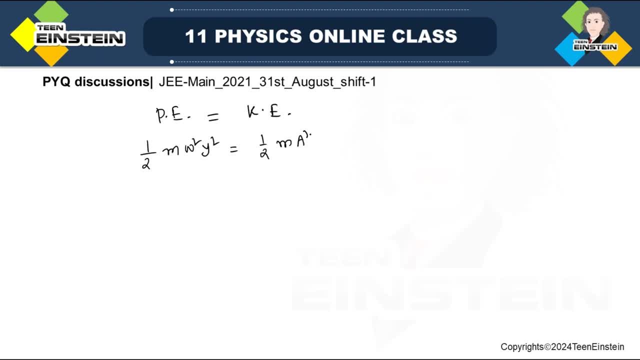 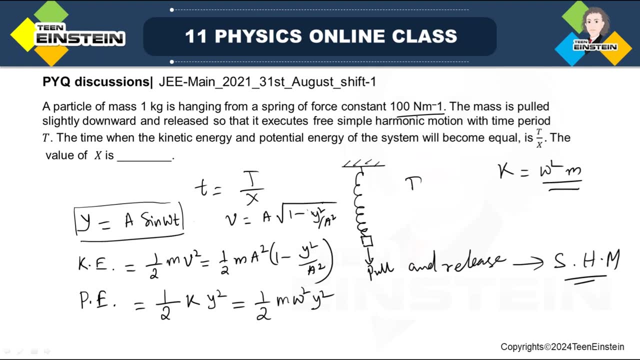 Yes, Okay, So I can write this. Yes, I can write. Yes, Okay, So the potential energy is equal to kinetic energy. Yes, Okay, Yes, Yes, Yes, omega into a, so that will be omega square. okay, so omega square. 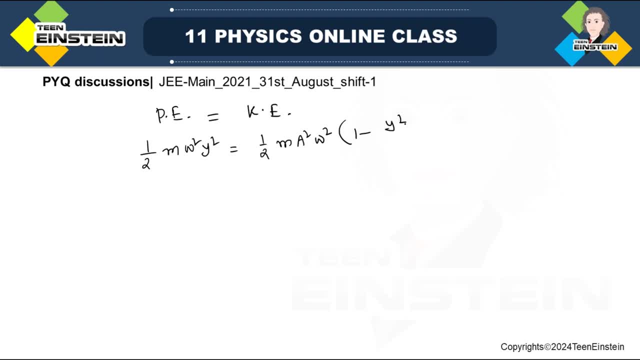 omega square whole into 1 minus y square by a square. okay, look then i will have half m omega square y square, physical two, half m a square omega square, this part along with half m omega square y square. okay, so this is the. okay, so this is the. 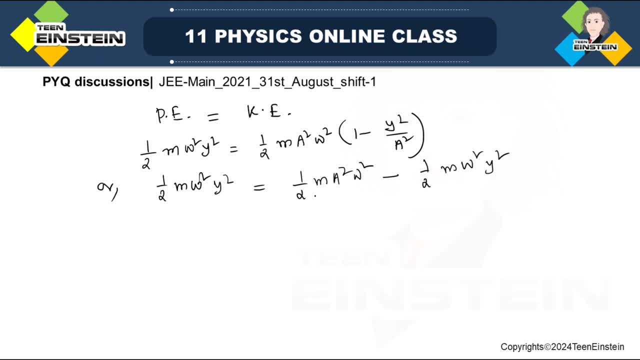 two. so these two i'll just take together so that i get m omega square, y square, and that is is equal to half m a square omega square. okay, omega square, m omega square. i can cancel from each other, then what i get, y is equal to the displacement at which the potential energy and kinetic 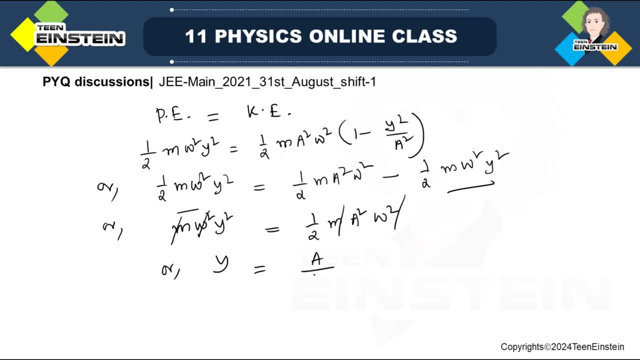 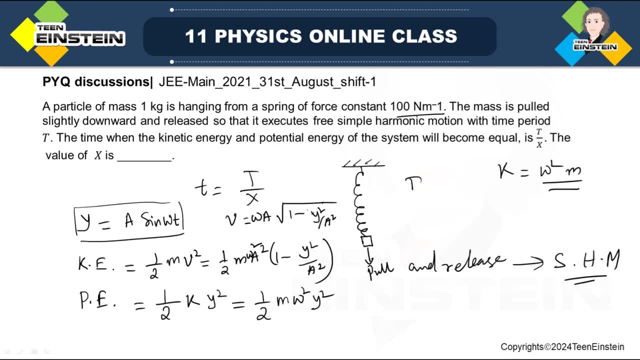 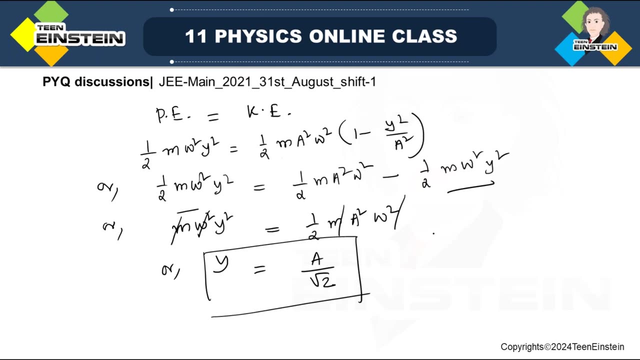 energy will be equal, is becoming c, is becoming a by root 2. so this is the displacement. see in the beginning itself what i have written as displacement. y is equal to a sign omega t. so let me just put it here. so y is equal to sine omega t. 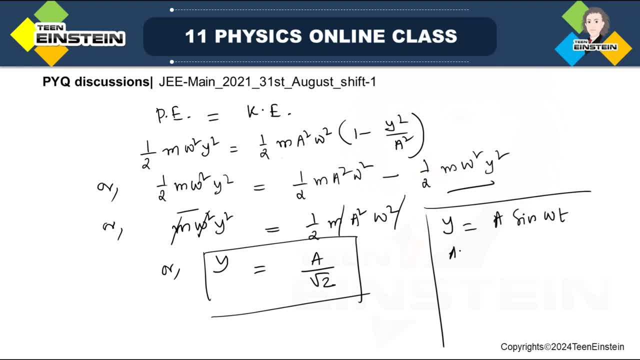 see, if I put this here, a by root 2 is equal to a sine omega t. then I get a sine omega t is equal to 1 by root 2. ok, that means, you know, sine omega t is equal to sine of pi by 4. 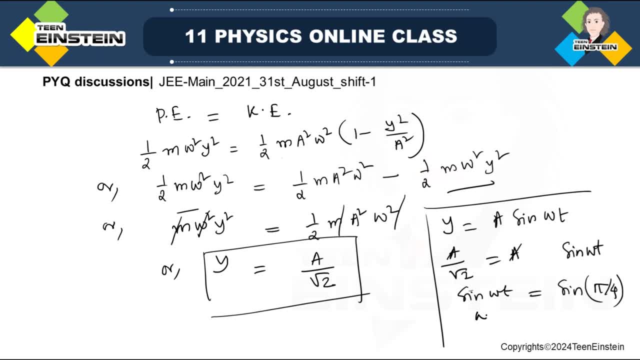 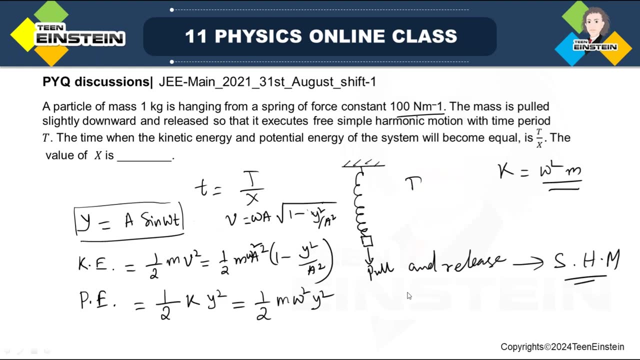 ok, so omega into t will be actually pi by 4, so from here I can get the t. look how so t will be. I think I have to claim this portion somewhere. ok, let me just put it here. let me write it here. so we have got omega into t. 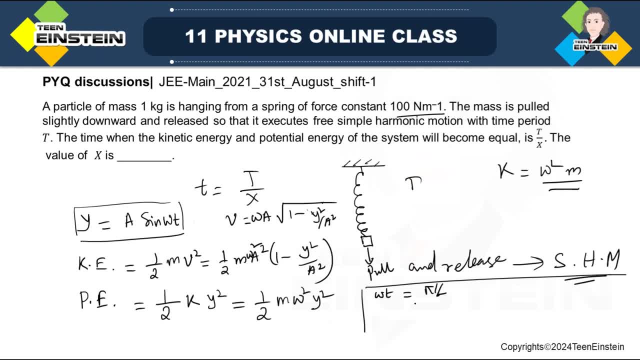 is equal to pi by 4. right, and see this. t will be pi divided by 4 into omega, again omega. we know omega is equal to 2 pi by t. ok, 2 pi by t. let us write that. so pi by 4 into 2 pi by t. 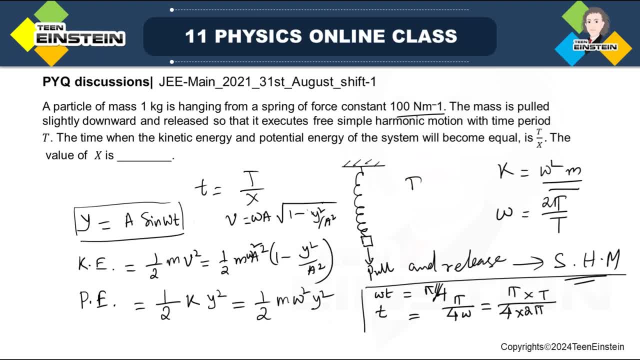 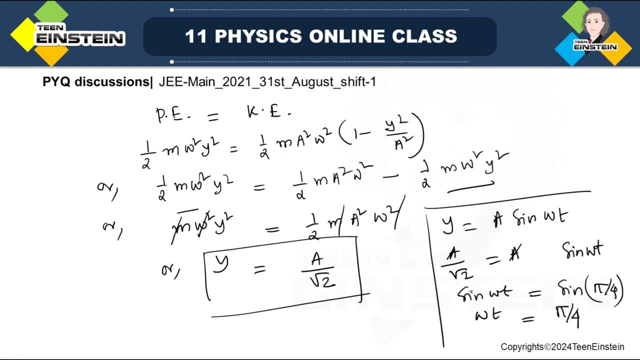 that t I can take in the numerator. ok, this will cancel each other. so t by 8, ok. so, dear students, look what I have done. I have actually found out what is the displacement at which the kinetic energy and potential energy are going to be equal. now, in this: 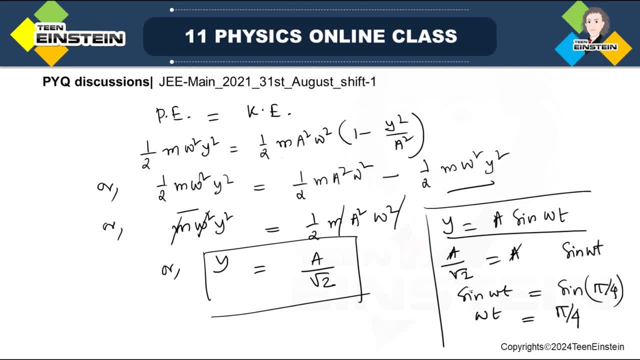 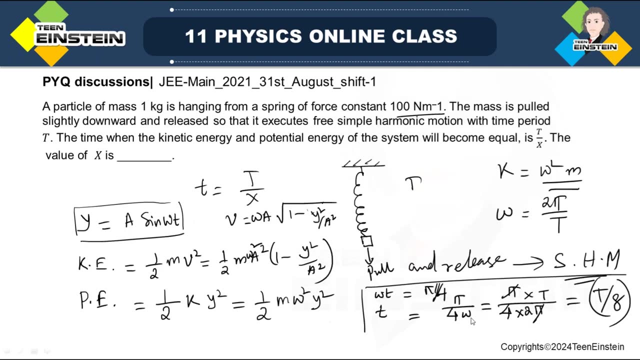 formula or in this equation. I am just putting that displacement so that I get a relation between t and small t, time and the time period. okay, so Omega T is equal to pi by 4. I have got. and then I have just substituted Omega in terms of T. okay, 2 pi by T. so I have got T by capital. a sorry, here the. 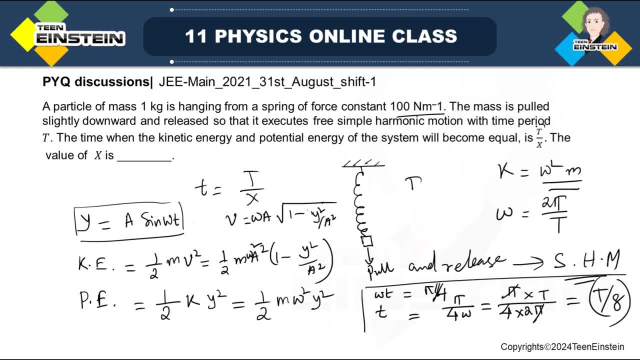 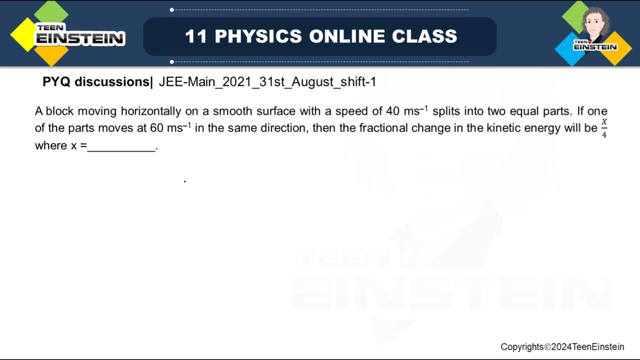 capital T, that is the time period by 8. and here, if I compare with this, then I get: X is equal to 8 and this is the answer. okay, so this was also a good question. now let us go to the next problem. see, here the problem says a. 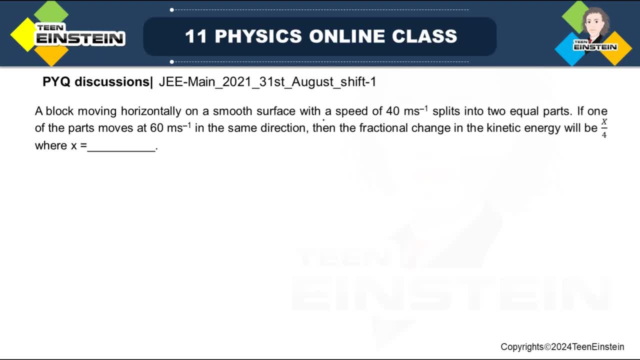 block moving horizontally on a smooth surface with the speed 40 meter per second splits into two equal halves. okay, equal parts. if one of the parts moves at 60 meter per second in the same direction, then the fractional change in the kinetic energy will be X by 4. fractional change in the kinetic energy. let me just explain the. 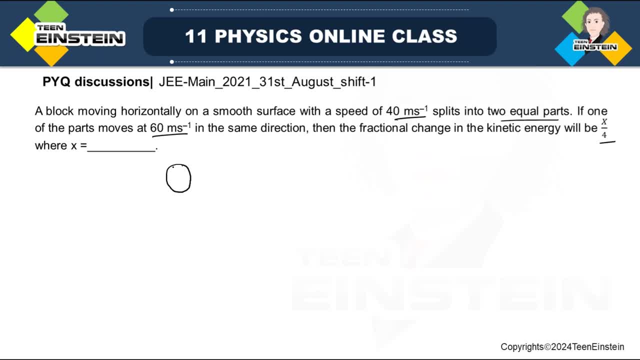 problem. see, suppose there is a mass like this. let us take this mass to be 2 am. it is moving, initially with velocity 40 meter per second. now, on the way, somewhere, it actually breaks into two. one goes like this and the another one, we don't know in which. 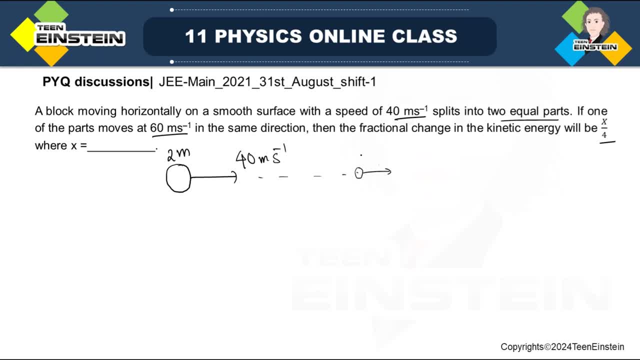 direction it is going. we'll just check it. okay, so it is actually. see, it breaks into two equal masses. so it is M and this is also M. okay, now this guy is moving with 60 meter per second. we don't know. let me take the velocity of this guy to be V. now the fractional change in. 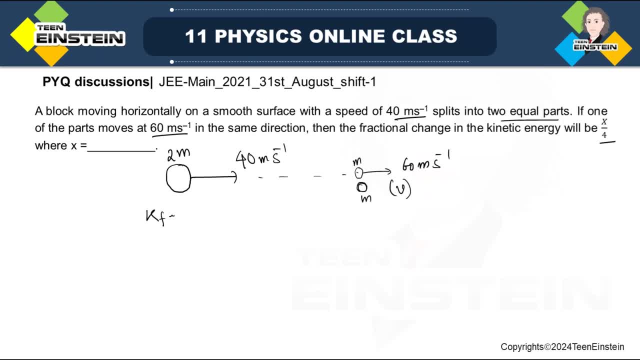 the kinetic energy. that means K F minus K I divided by K I. this is actually fractional change. this can be mod. okay, this is fractional change and that is given as X by 4. okay, we have to find out. what is this X? so here, anyway, let us find out this velocity by applying. 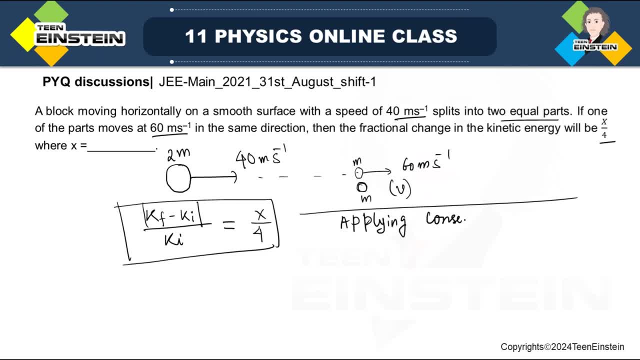 conservation of linear momentum. conservation of linear momentum, of the linear momentum. okay, so what is the initial momentum? that is 2 into 2 m, into 40 meter per second. so it will be actually so. this is initial momentum. this will be 80 M. let us take that as K Z. 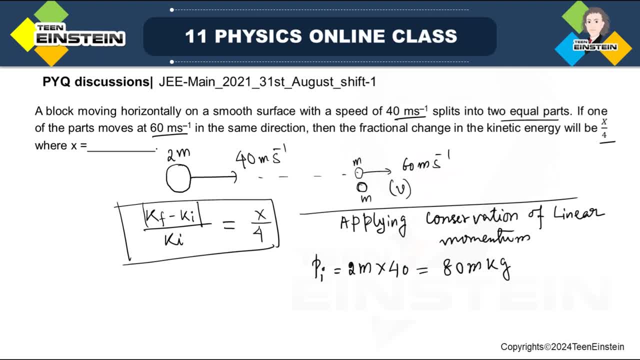 K, Z. so okay, so this M will be there because I have taken 2 M. so that's how M is that Casey meter per second? okay, but what is the final one? so final one will be M into 60, so 60 M plus M into V. I'm just taking as plus and 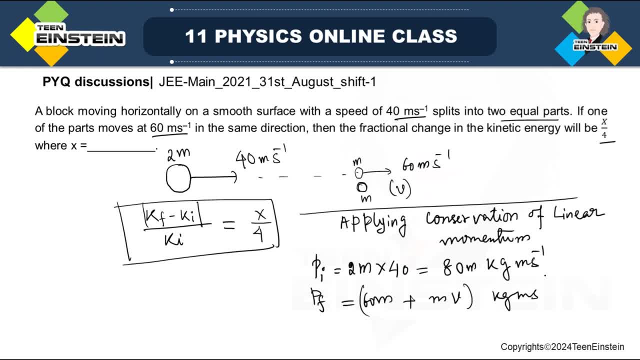 so this is also in kg meter per second. so these two will be equal, okay, linear momentum, in any case, will be one chart. okay, if i just do that, then see what i get. i get m into 60 plus v is equal to 80 m. okay, so from here this m, m goes off. so we, we get actually. 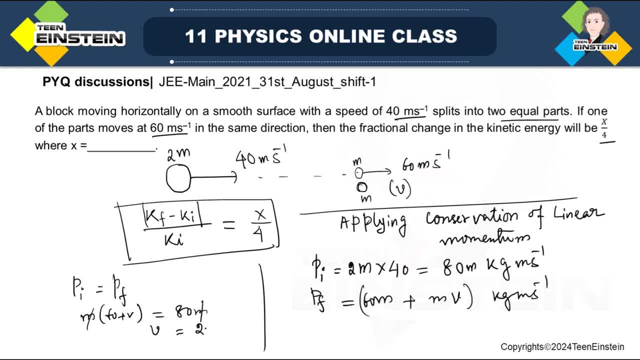 60, so 60, 80 minus 60, that is okay, this is 20 meter per second. so other one is also moving in this direction, in the same direction, because the positive sign is positive. so other one is also moving in the same direction with velocity 20 meter per second. okay, now we have to find out what is the final. 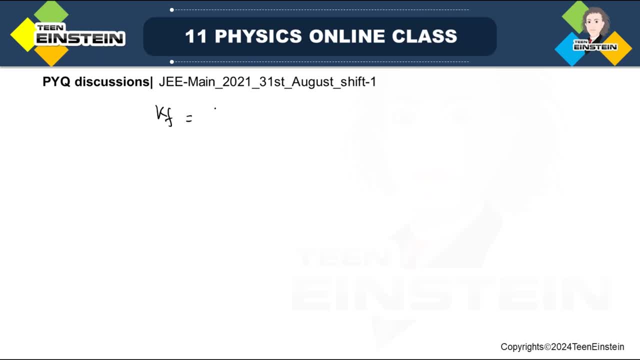 and initial kinetic energy. so final kinetic energy will be half m 60 square plus half m 20 square. okay, so this will give. you see, this is uh 30, so 36 800 m and this will be 200 m. okay, this is actually kinetic energy in joule or whatever you say. so this will be actually 2000. 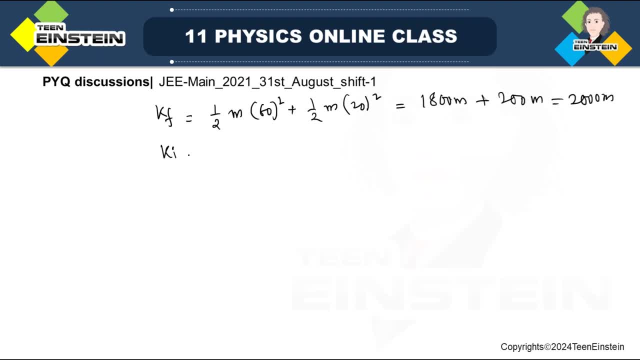 2000, a. what is initial kinetic energy? that is half m. m is 2m here into 40 square. so 40 square is actually 1600 and divided by this, okay, this is actually 1600 in. okay, so let us find out the difference. delta k is kf. 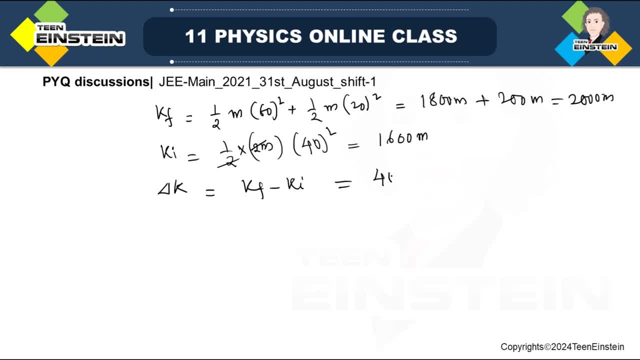 minus ki, that is 400 m. what is initial one? initial, we know. so we will get fractional change, fractional change in k kinetic energy equal to 400 m by 1600 m. that is the initial one. so you get one over 4. okay, one over four, so let 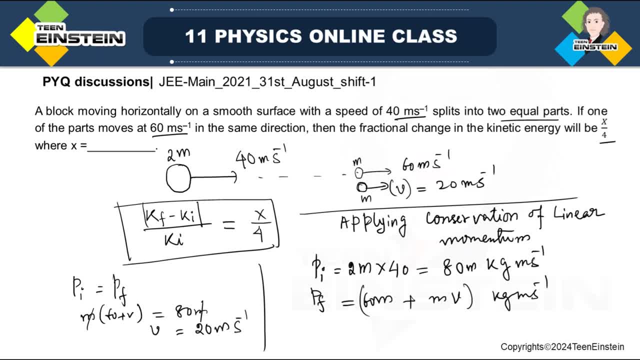 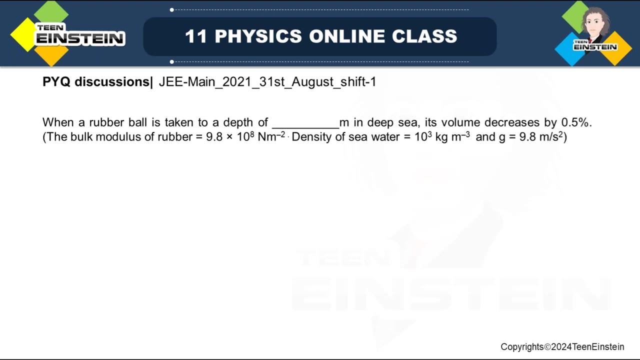 us compare with this one, so this is x by four. that is compared with 1 over 4, so x is equal to 1. so in this case the answer is one. okay, okay, let us go to the next problem. okay, so this problem says when a rubber ball is taken. 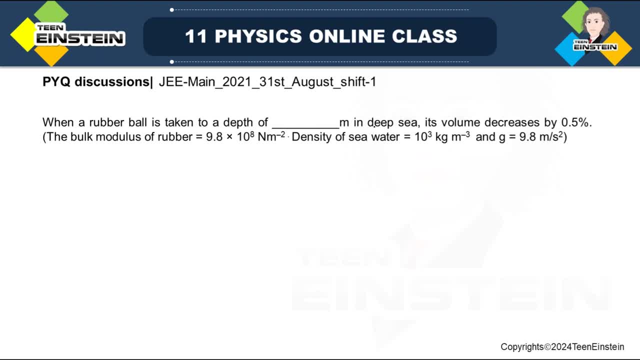 to a depth of dash meter in deep sea, its volume decreases by 0.5 percentage. okay, that means you know the delta v by v. this is in percentage if you multiply 100, so you will get in percentage. okay. or we can say delta v by v is 0.5 by 100. okay, so this is given here. 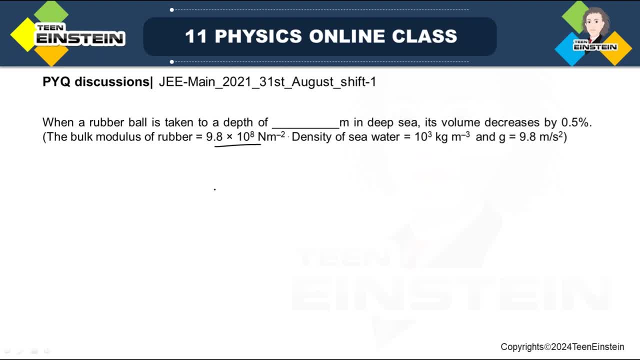 the bulk modulus of the rava is given, that is 9.8 into 10 to the power, 8 newton per meter square, and density of the sea water is also given, that is thousand case per meter cube, and g we have to take as 9.8 meter per second square. 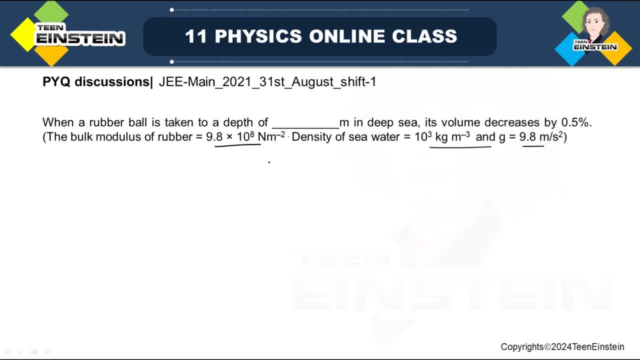 so we have to find out what is the depth we have to take. it see, bulk modulus of the rava is given right. let me just find out what is bulk modulus actually? bulk modulus k is minus del p divided by del v, by v. okay, this is actually my bulk modulus, so let us just 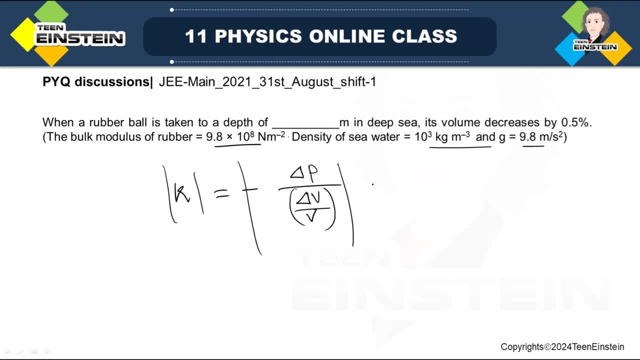 take the modulus. okay, so we get delta p by delta v by v. okay, so this is actually my bulk modulus. k is minus del p by del v by del v. so if we consider with respect to the sea level, so this delta p i can write as h? rho and g. okay, h rho, g. so from there i have to. 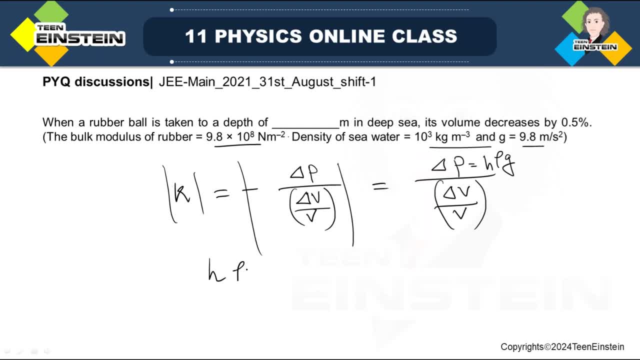 find out. what is this h? so h rho g is equal to the bulk modulus into delta v by v. okay, so from here h is equal to k delta v by v, divided by rho into g. so let us put the values 9.8 into 8. this value is unit less, so this is 0.5 divided by 100. 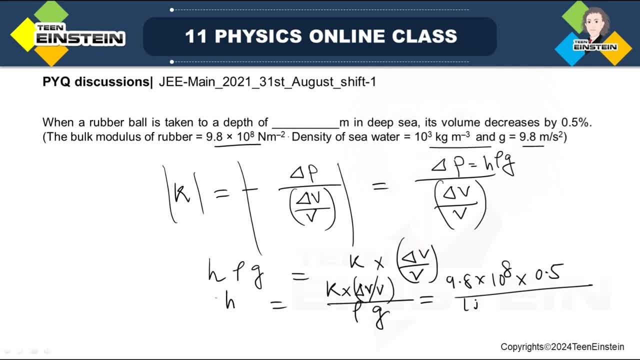 now, if we want to put g over here, we have also to take in g as 0.1 into 1 by 2 and the Snyder curve here. this is g x 1. we are not targeting g x 2. instead we will be using this.